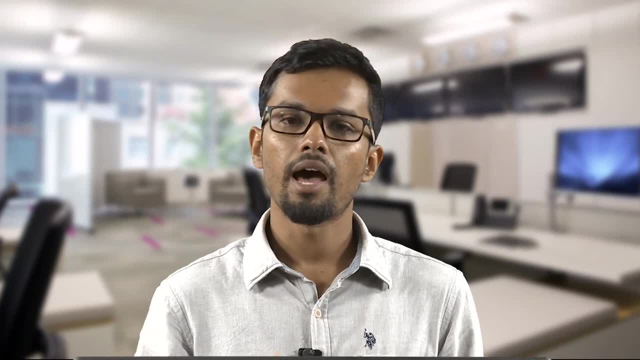 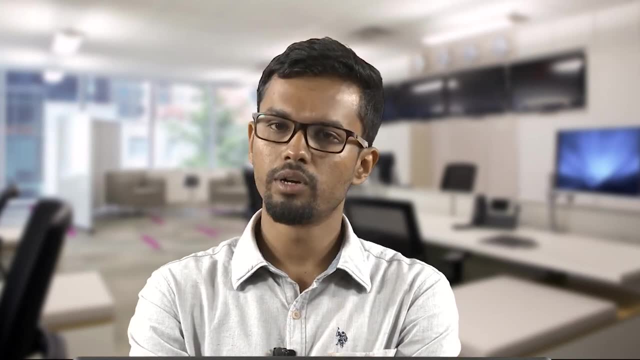 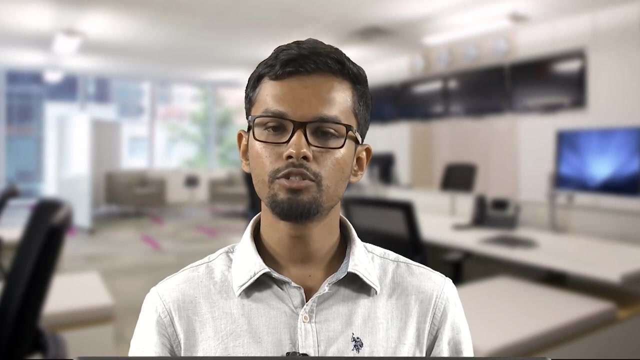 the feedback and this kind of falls within a loop And unless and until the final product of the website or whatever interface is designed which satisfy the user, that does not launch the market. So that is to ensure whether this product should not fail, because lot of money is involved. 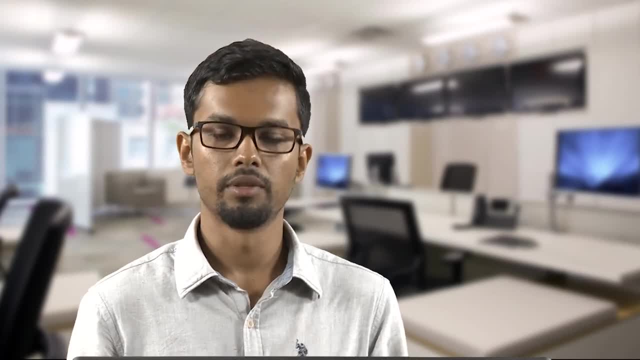 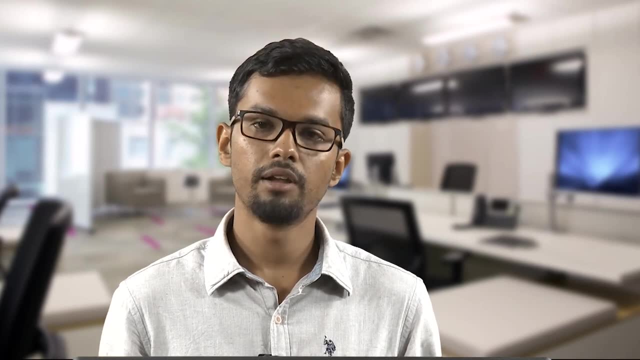 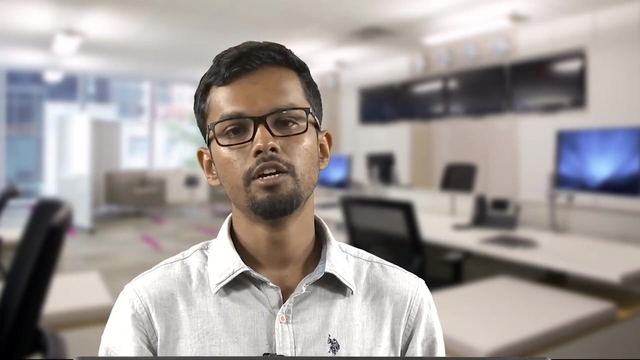 within the market launch of the interface. If we look at the web application of different mobile phone or the features of the mobile phone or any other devices which has an interface part attached with that, so that is fixed. when the product is launched It gets updated. the 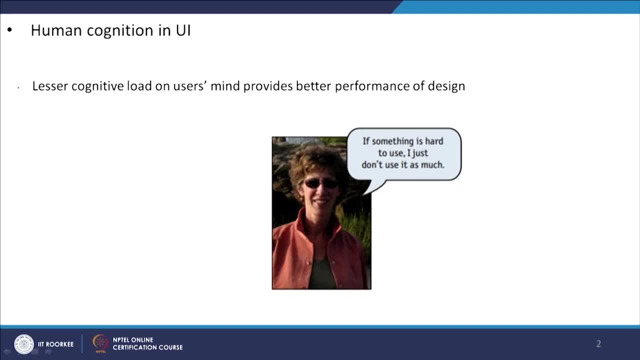 software or other things, but still lot of money will be already gone when it launches the market. So to ensure the failure, to ensure that product will not fail after launching the market, so it is important to adopt the iterative model of design And we have discussed many 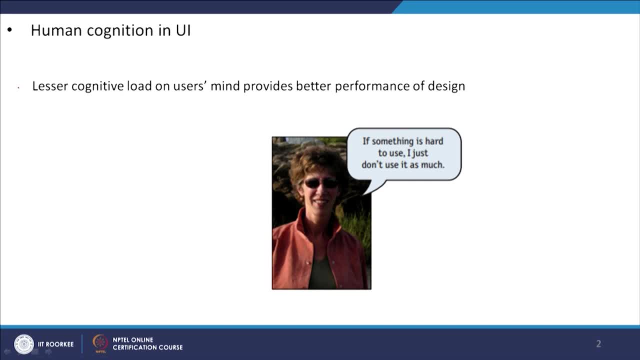 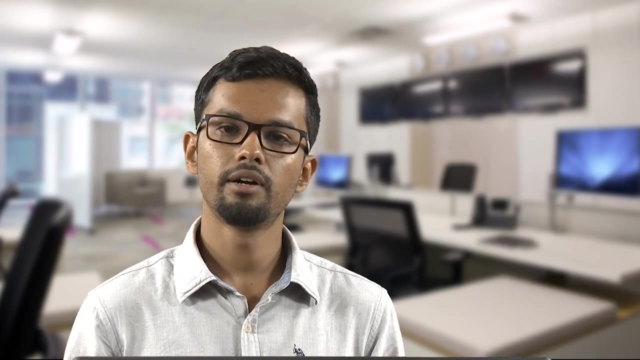 iterative models of design and, through Donald Rommon's double diamond method, six sigma design processes and design thinking frameworks. So all of this framework has a very important component, which is the users opinion into the design. So more and more we are going towards the new. 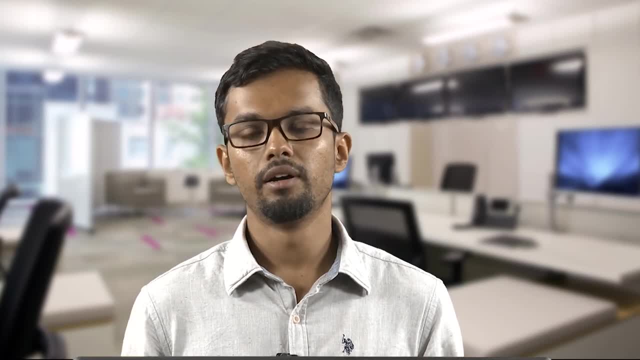 process of bottom up approach of design, where we start with understanding the user. So user s voice, so the voice of customer becomes very, very important. So let me give you some examples where we consider the user. So let us say I have a particular popup. 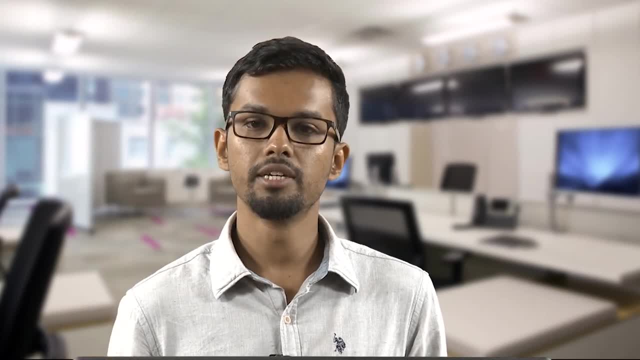 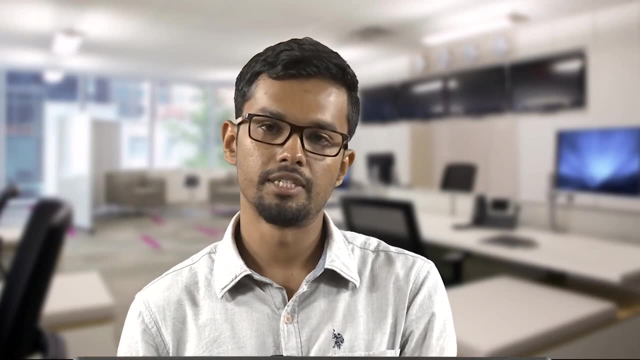 Sojoy could get milk and put milk in the cup Like acrid cereal can probably feed each of my options. So the the component here we will start discussing today will the importance of human factor into the interface design. So when we start discussing the design process we start with. 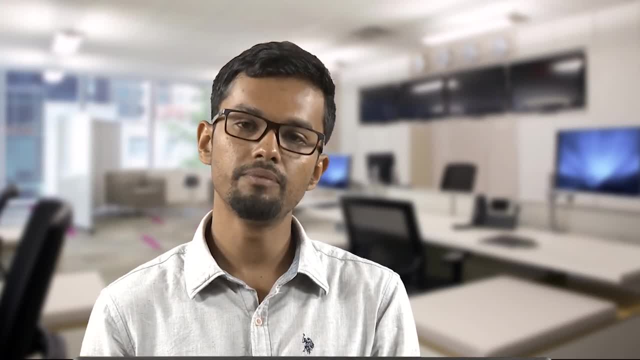 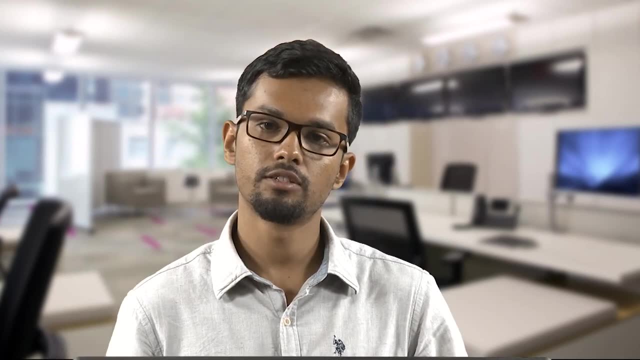 the user and finding their need. So that we also have seen in the previous design process, when we started discussing So human factor in the interaction design, why humans are so important, why understanding them so important. So if we do not understand the particular target, 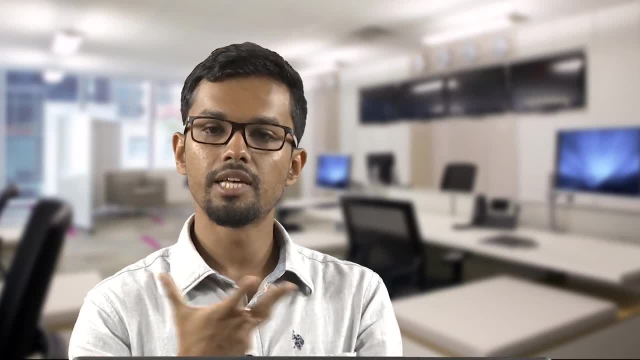 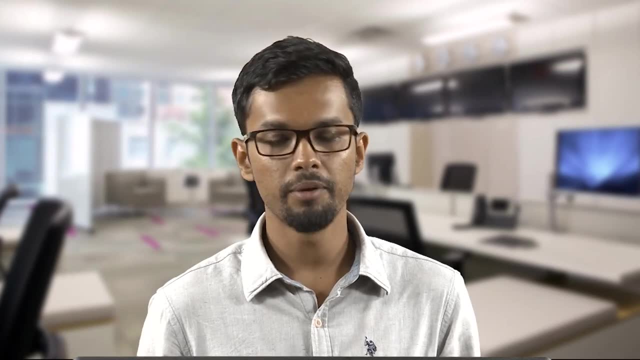 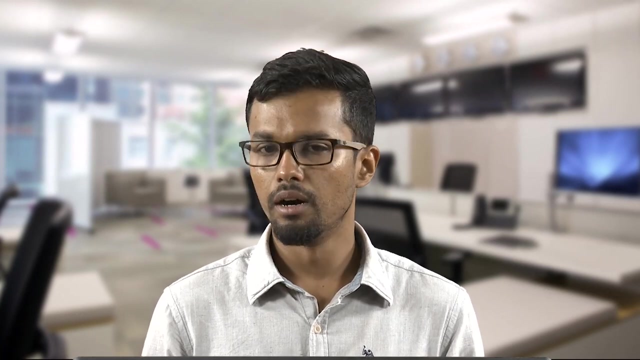 audience or our real customers need the design, and everything will be not successful when we start the next process. So the first process will be understanding the human s behavior. So few of the things which we will discuss later when we start testing and doing the study, but few of the human traits, how they. 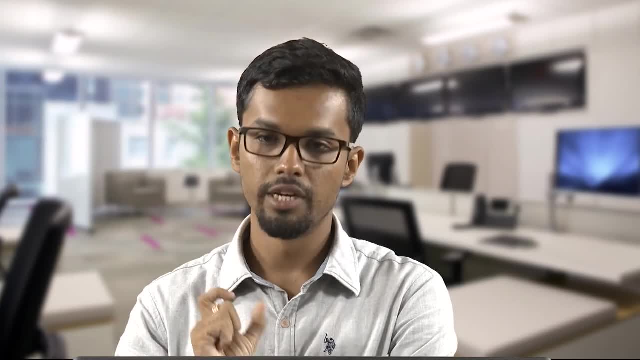 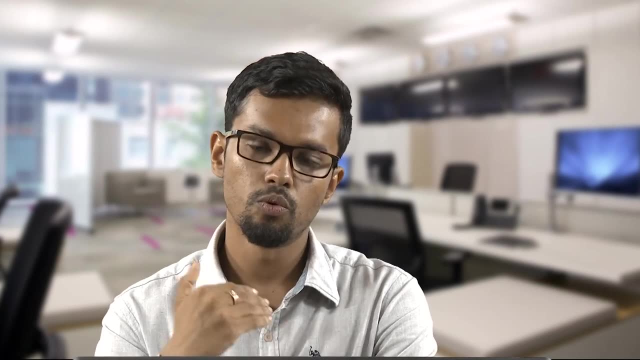 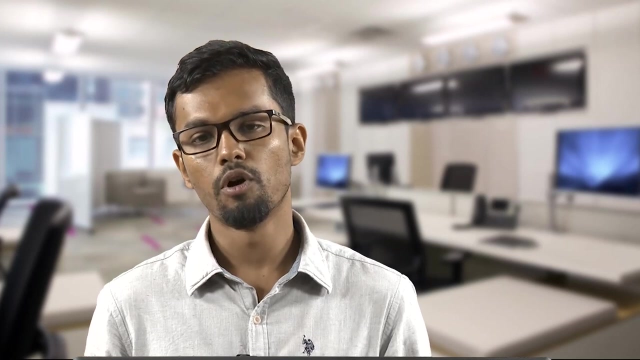 user interact with the interface. So here I am talking about the only the interface, how people interact with the interface, only in this context. So what are their probable psyche of the users? So that we will start discussing and then we will move on towards the next tools and techniques of 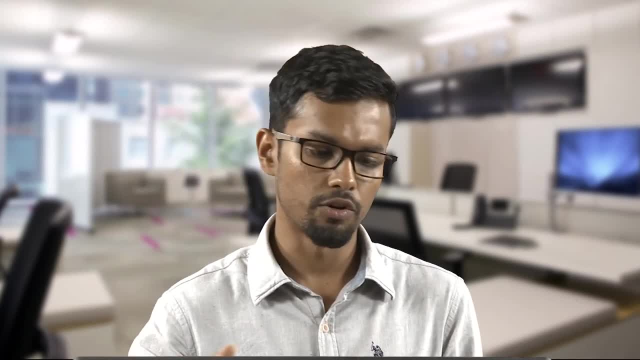 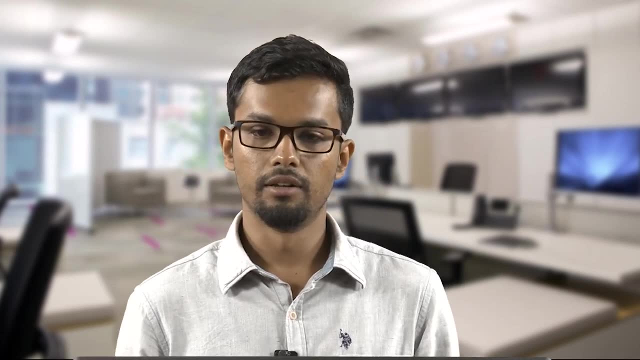 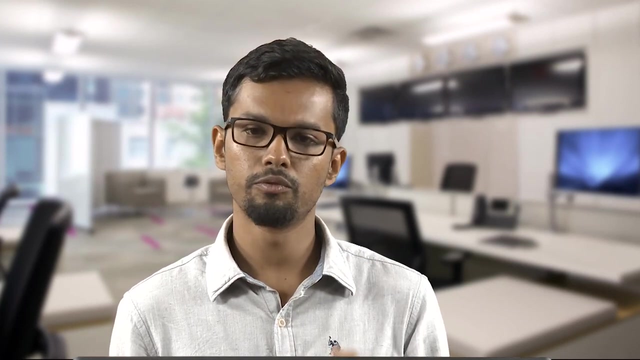 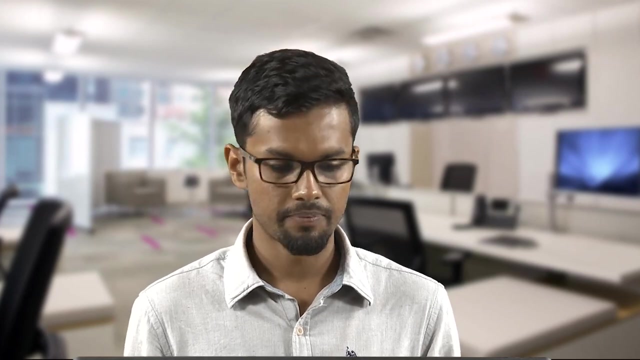 users study in the next class onwards. So first few of the myths, or it can be the how people behave when they interact with the interface. So what is the human factor component which is the most common factors of human behavior when they interact with the interface? So the first truth. 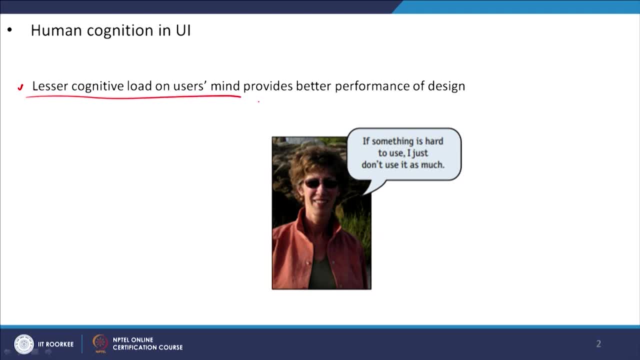 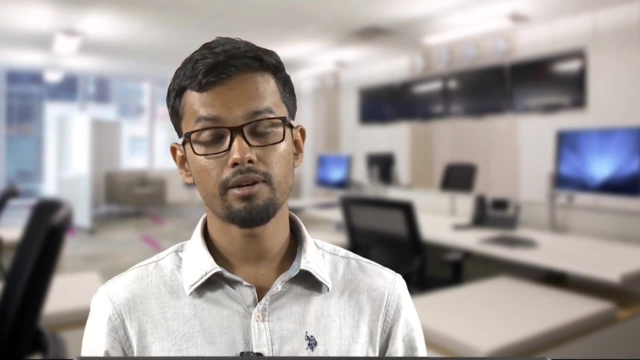 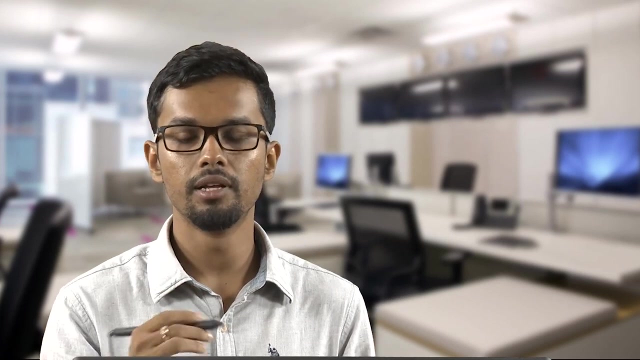 is lesser cognitive load on user's mind or user processing within their psyche will provide a better performance in the design. More we overload user s mind, that more the decision making processes, more question marks comes within the user s head. the users will be frustrated and users will not fulfill the 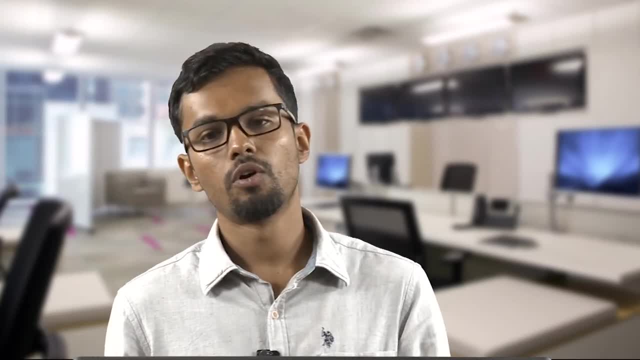 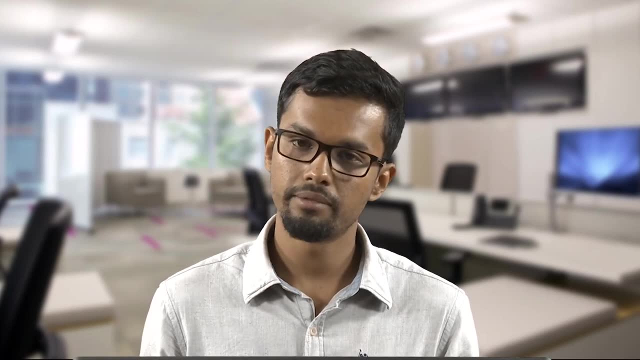 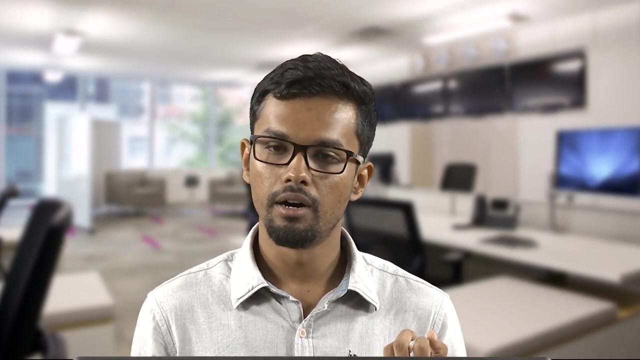 web application. Most of the web applications or the websites provide information and it might relate to some task, For example, if there is a e-commerce website, so they are trying to order something from the online portal, or if it is a train booking or hotel booking website. 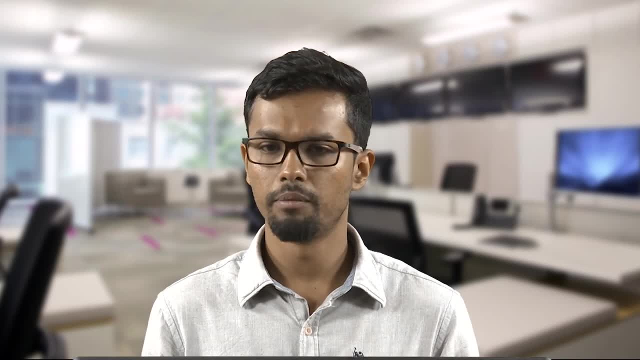 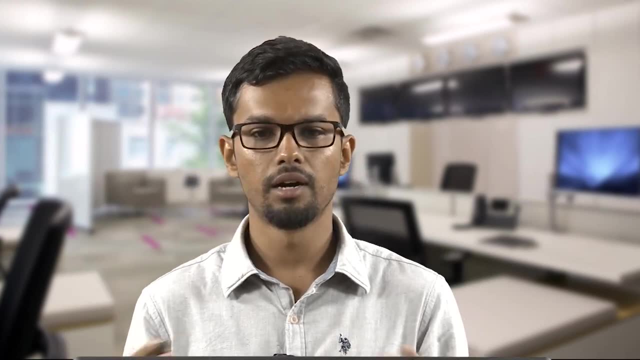 so they are trying to book something, or if it is performing any other options, for example chat, so they will try to chat with people and then other different website perform different, other jobs. So there is a task related to the user, So you will have to do some work. So there is a task related to the user, So you 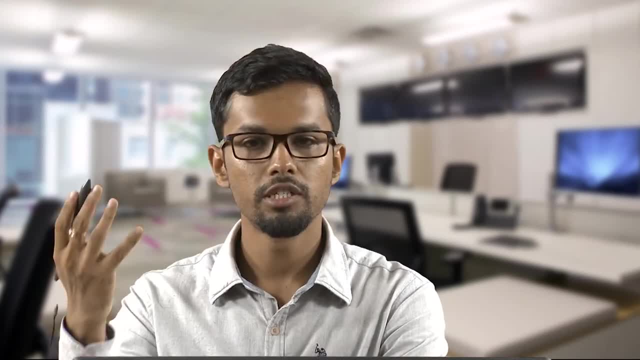 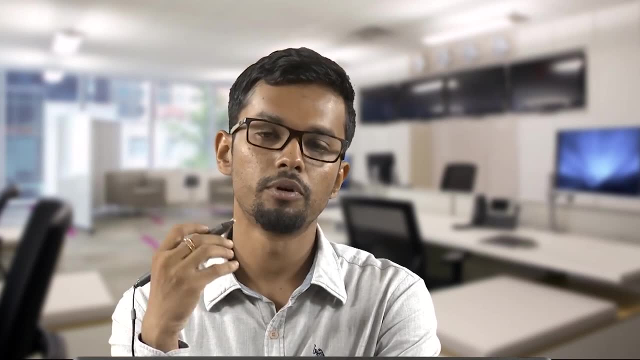 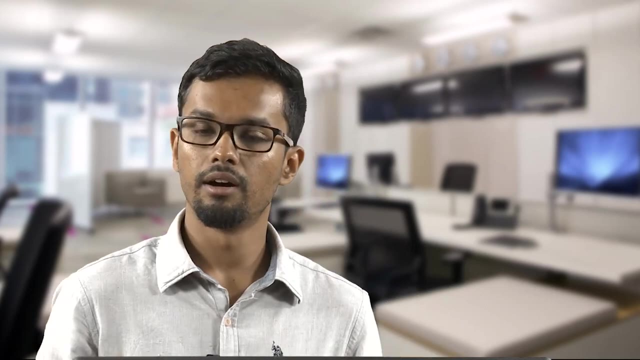 have to perform a task. So, based on the information which is given within the website, these informations in the websites are telling the user to perform the task and what kind of task they can perform using this website. Users are trying to grasp while looking at the button. 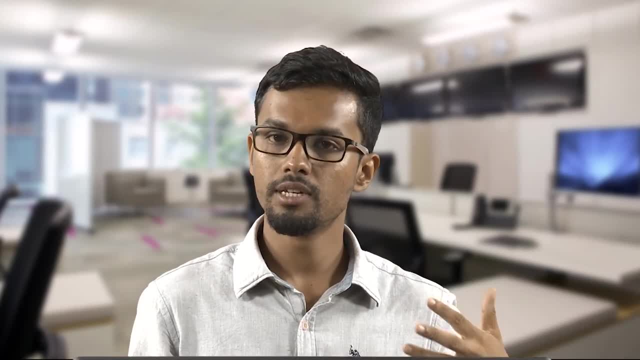 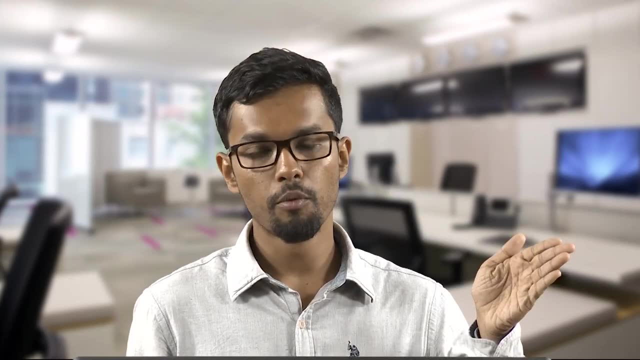 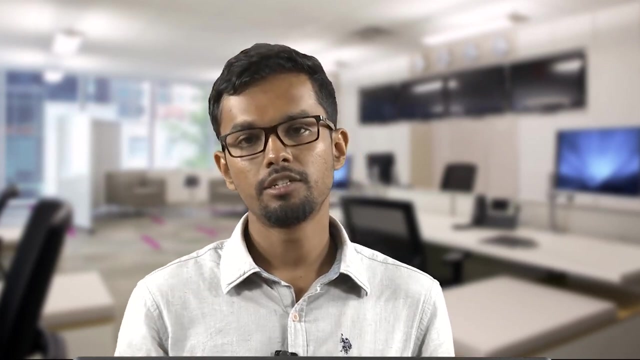 And then users also have some process within their mind which is their mental model. So they have already thought about some kind of probable steps of the task. So if that matches with the website or web application, that will help them to do the task faster. The faster they perform the task. 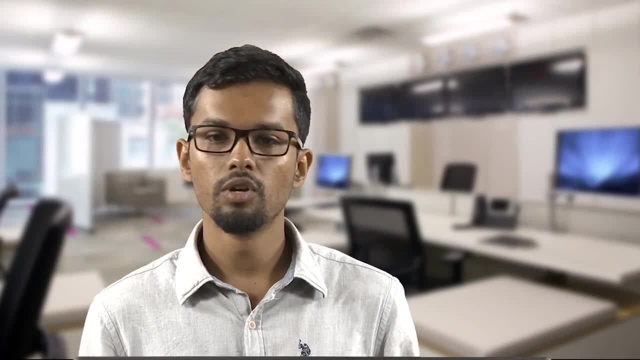 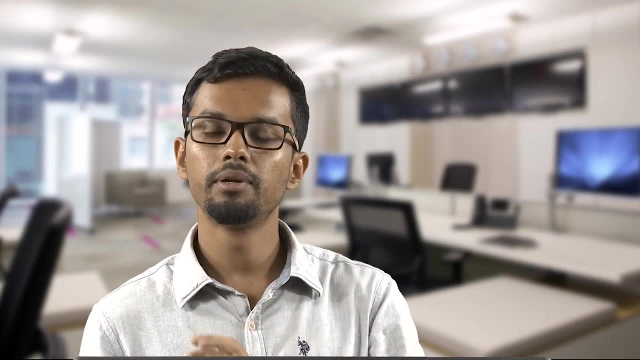 the more successful the website it is. So if they cannot even perform the task or it takes lot of time to perform the task, they will not visit the website. If there are multiple different other options, the market competitors are already available, So they can perform the task. 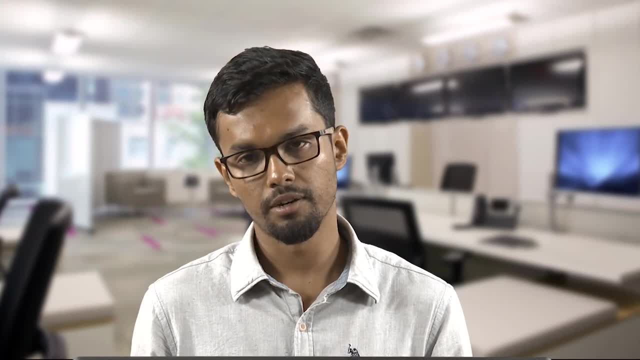 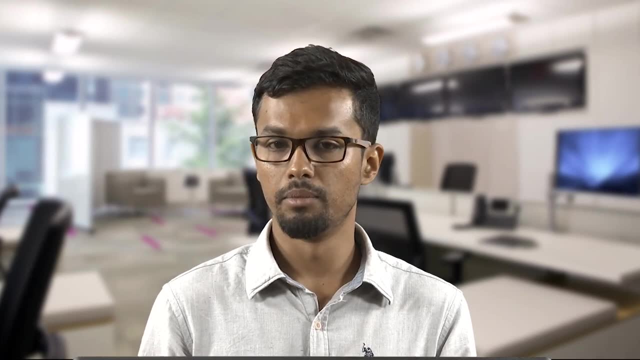 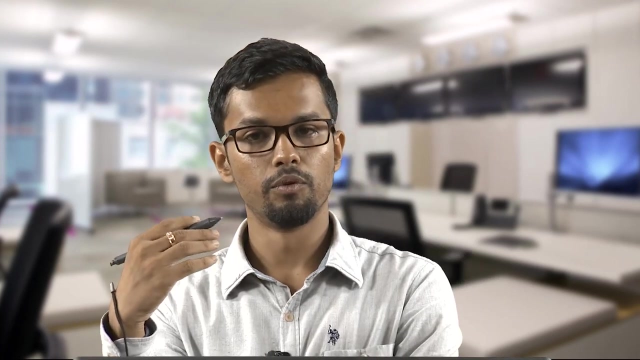 So the website will lose its potential customer and the advertisement which is there in the website will also not fetch the money and potentially it will not be successful. So, more and when users will perform the task faster when there is a lesser processing or the lesser cognitive load. 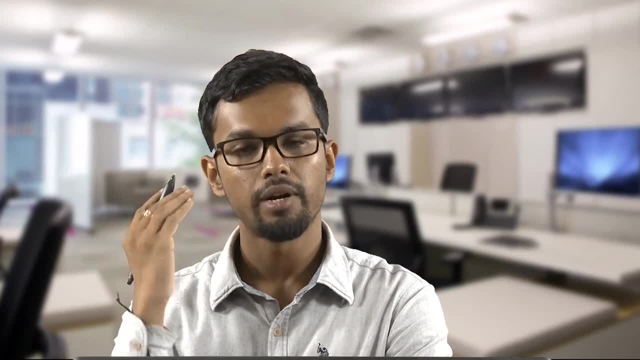 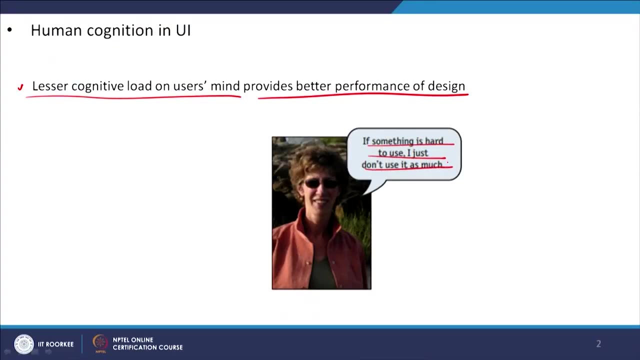 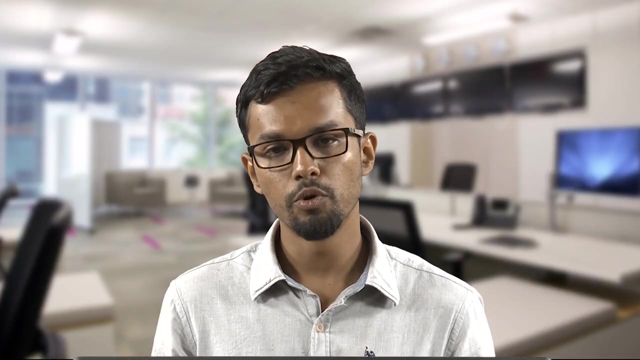 is there So they quickly understand what is the task and how they can perform the task. So if something is hard to use, this is how common users will say. This is taken from one of the famous book in UI UX design, which is Don t Make Me Think, by Steve Krug. You should go read. 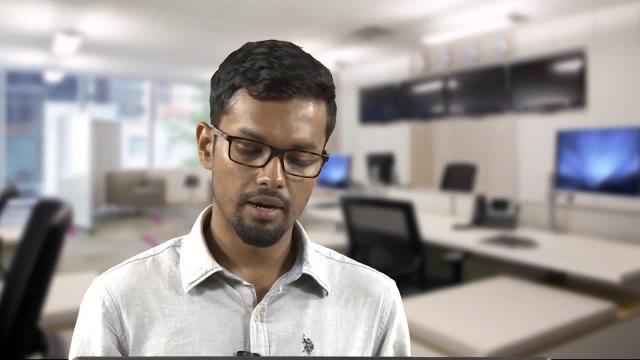 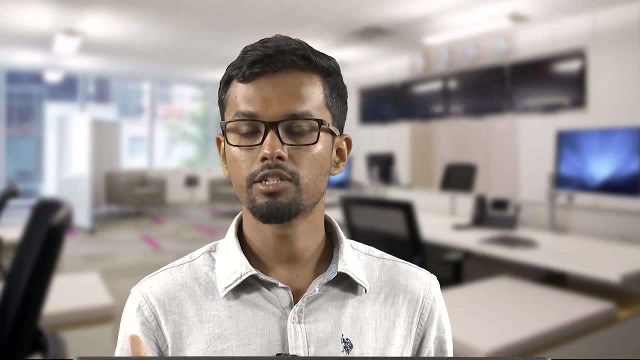 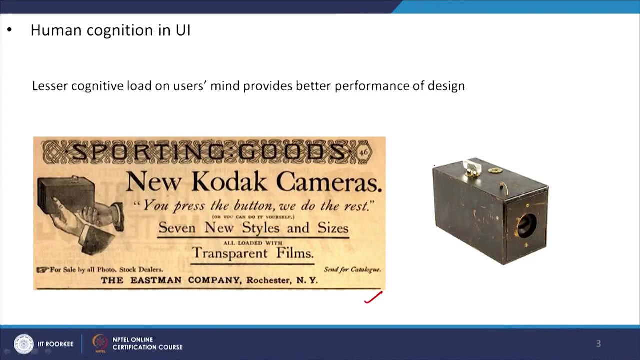 that book in your spare time. So the user s common behavior of a user is like: if there is some task is something, some product, or it can even be the interface is difficult to use, users will not just use it. So this is the product launching caption of first Kodak camera. This is the first Kodak. 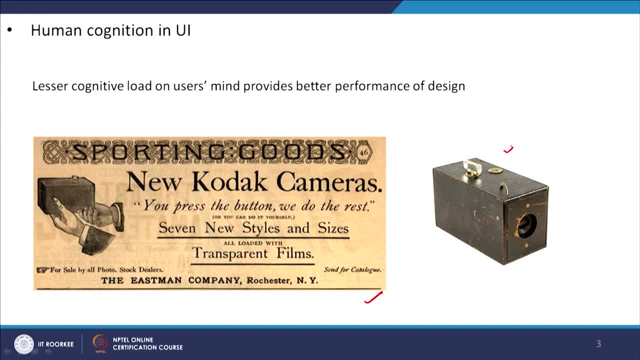 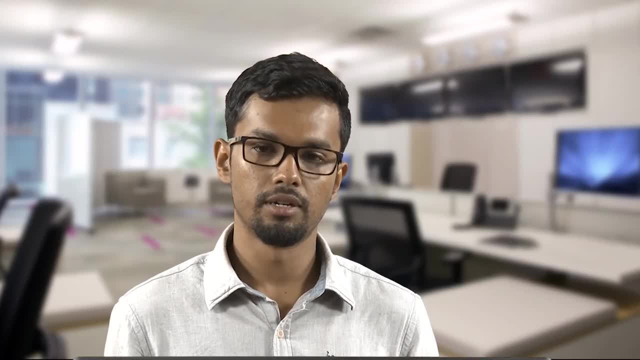 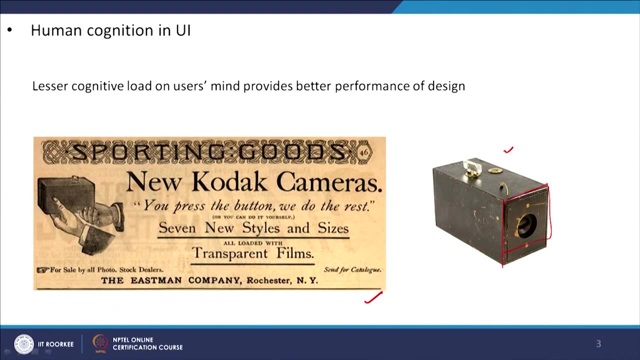 camera for personal use. Before that there was bigger camera, So this is for people s personal use. After industrial revolution, this boom in the product design, this is one of the outcome for that, And so you can see the internationalist style, the minimalistic. 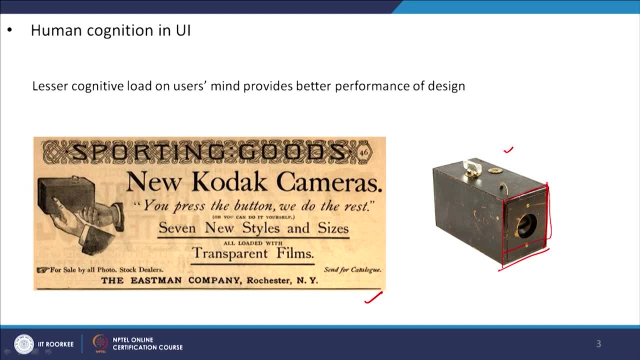 style is there that is different, but the main thing is how they wanted to portray this product. So they are writing that you press the button and we do the rest. So they are trying to emphasize that the new Kodak camera, how the main feature of this- 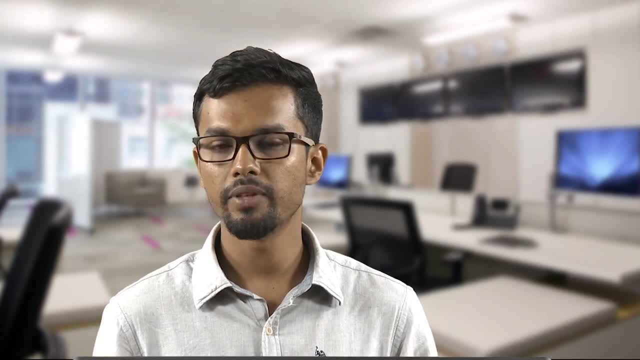 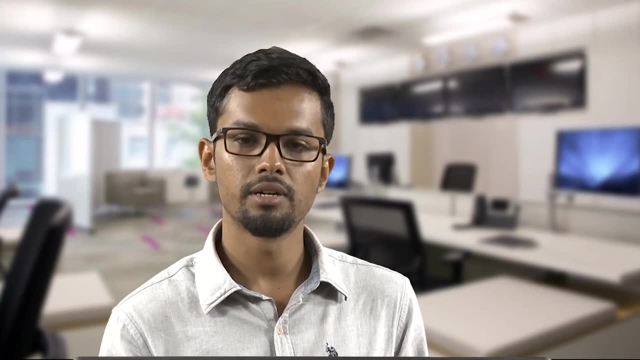 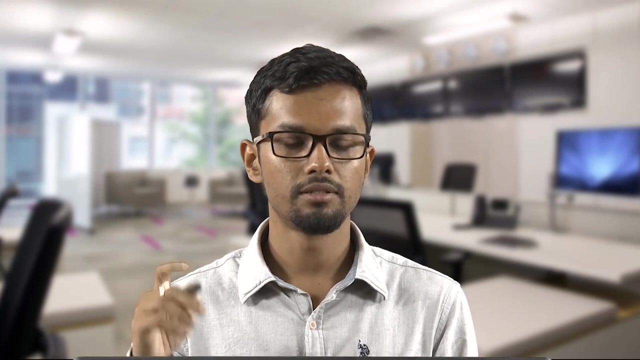 is you just press the button and rest. everything is like a black box. What is happening within the camera you do not need to know and you get the best result and the best picture comes out. So there is no different process. There is just one process: you click the button and this is the function is done. 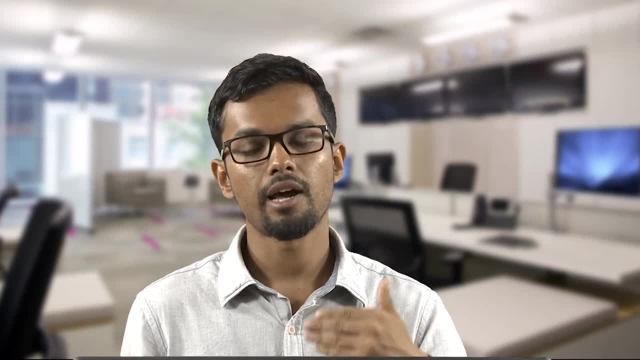 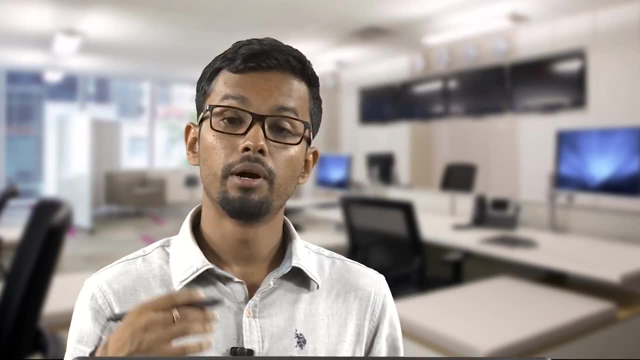 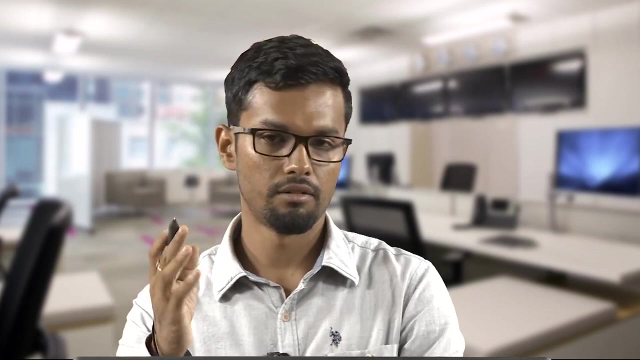 So they are focusing on the ease of use, and that attracts the users the most. So if the product is easy to use, users will be happy, But on the other hand, users want more and more features. So there is an optimum balance you have to perform. 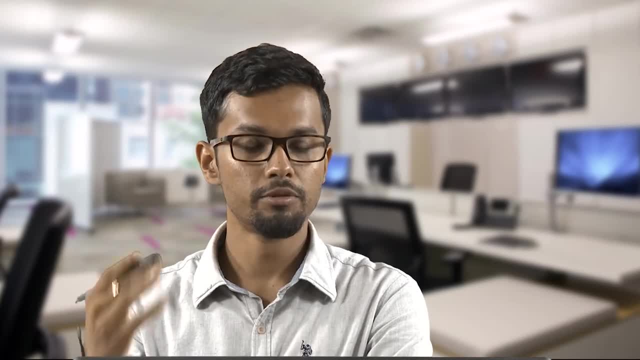 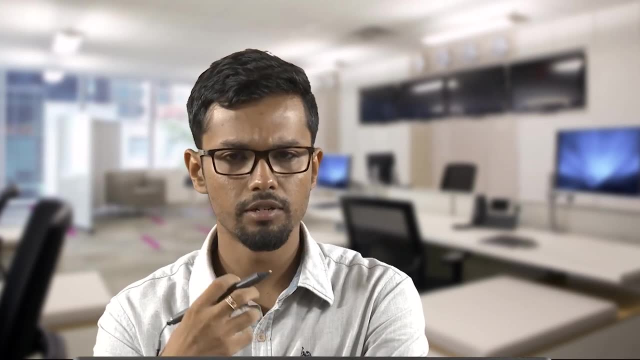 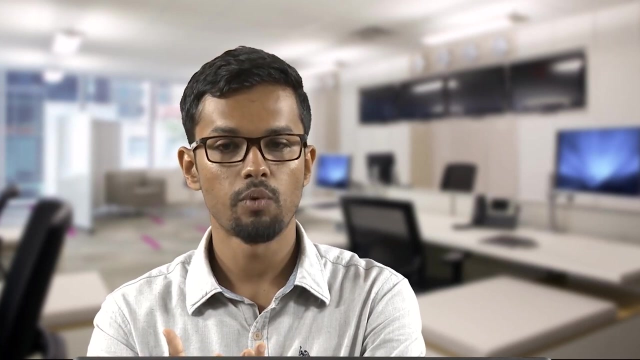 So even in the website. so user wants the website to fulfill lot of task they want and each and every task should be very quick and lesser the number of steps for each and every task is convenient for them. So they want multiple options at this one side and users want and then they want these. 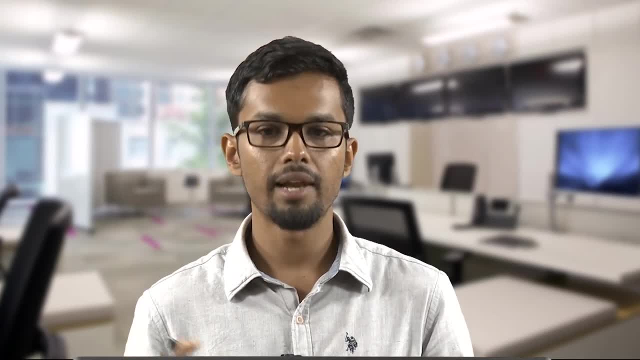 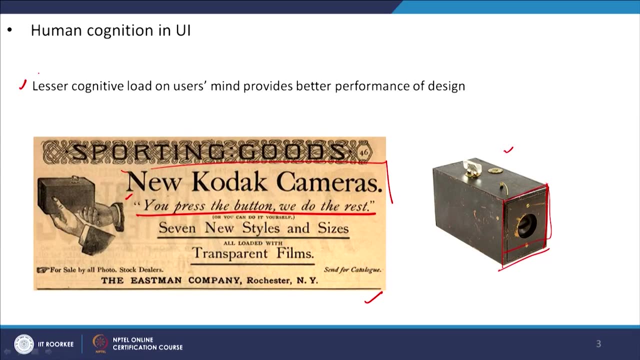 options or the task to be quickly fulfilled. So there is a balance has to be drawn from the designer side. So the main thing, The main thing is here: when in this point which I am trying to mention is the lesser cognitive load, quicker the process of one particular task, better it is. 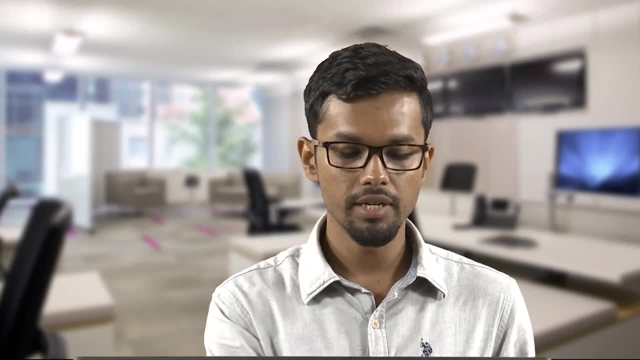 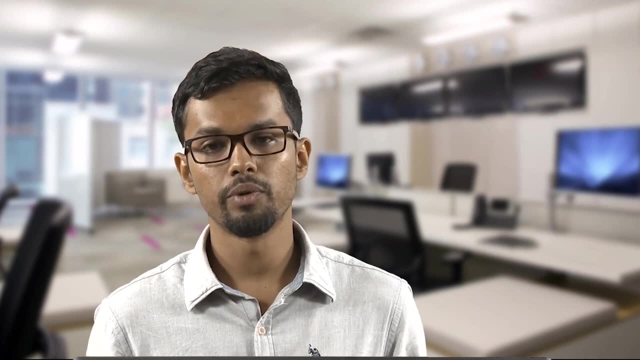 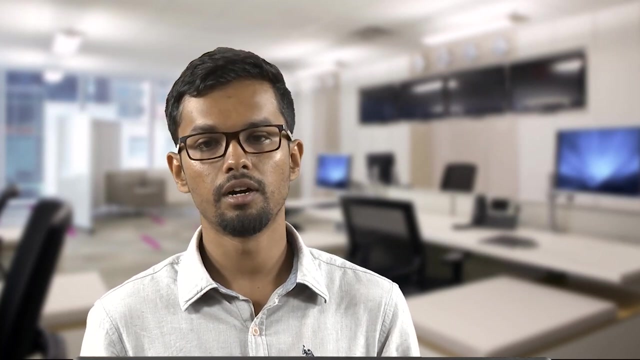 Next, to achieve this most obvious answer over doubts is has to be designed So there can be multiple. when we create multiple ideas, when we think about multiple solutions, there can be different ways to represent the fulfill the task. different terminologies can be there, different type of information can be there. 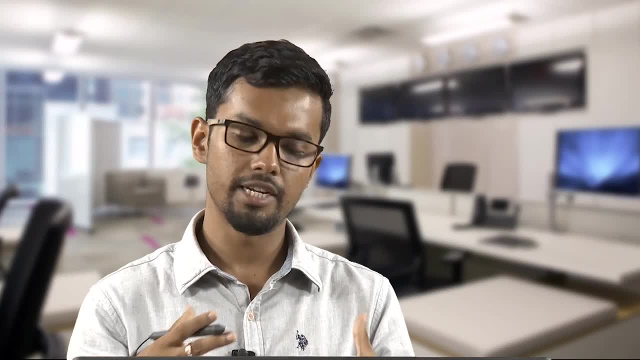 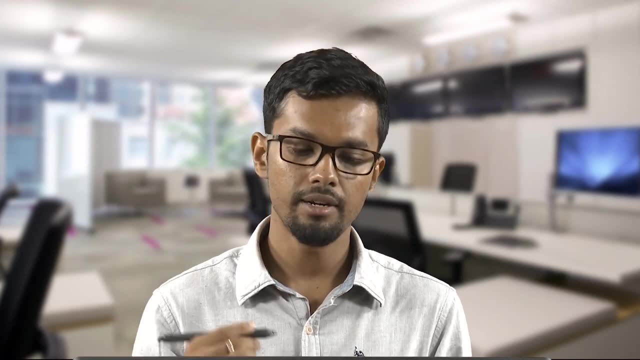 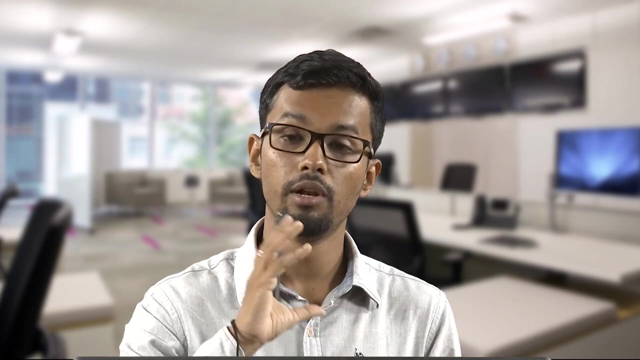 But when we are segregating, we are converging to one idea. then we should look towards selecting those options which is more obvious than those option which can create a doubt within users mind. So they will, if they are not sure about how this. if they click on the button, what will? 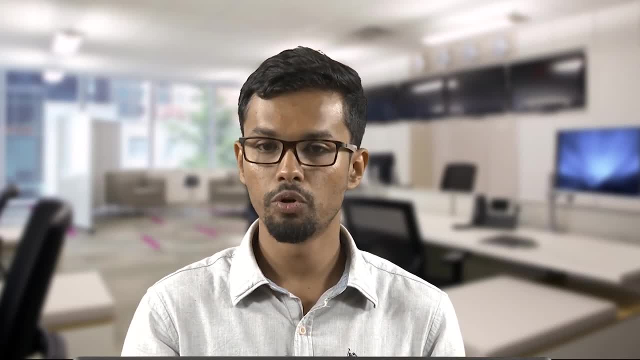 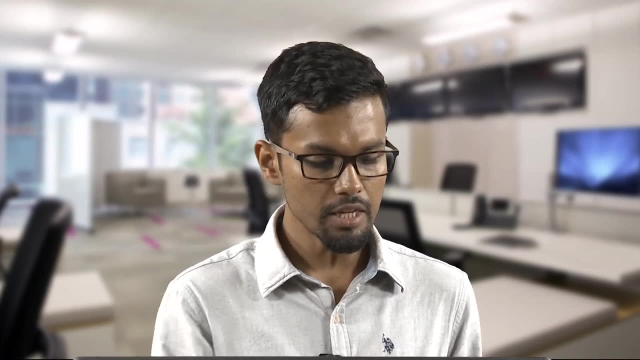 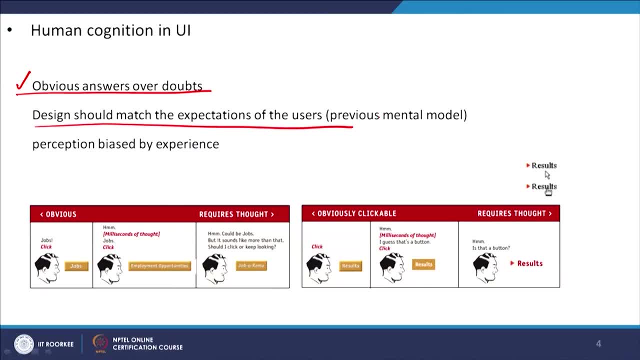 So design should match with the expectation of the users. So always, user have a mental model. So whenever users are exposed to a different product, they will create a perception about the other product which they are using. So this can be based on because they have already used similar product or if they are. 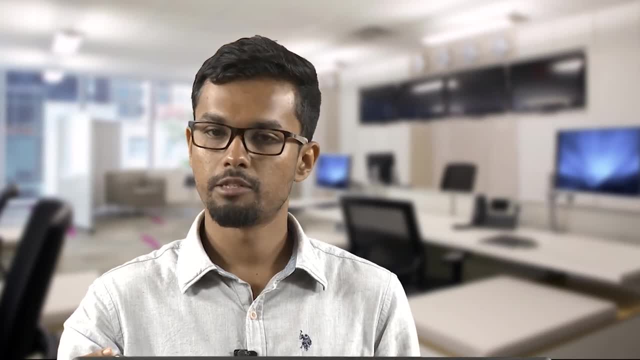 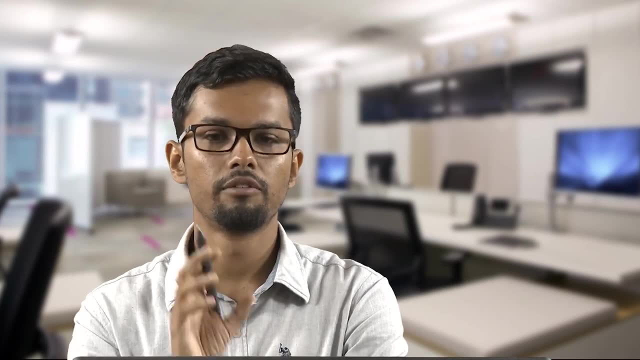 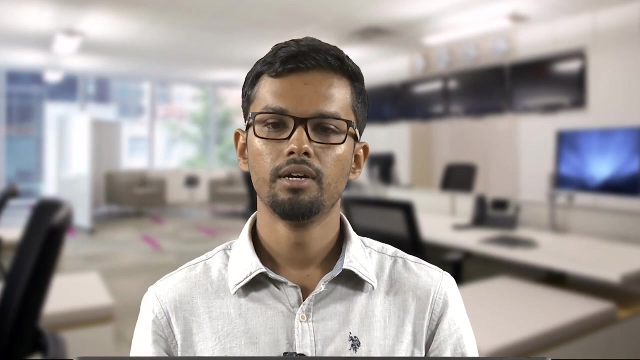 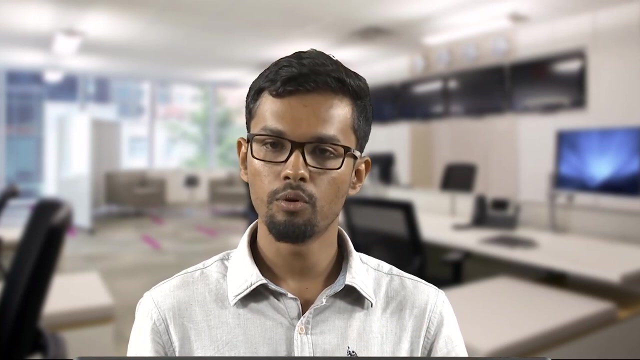 not using the similar product. still based on their previous expectation, they will have a perception of the product in mind, So which we have discussed in the model of designers, conceptual model, customers, mental model and the system image, this stradic relation we have discussed. So, based on that, they have always a expectation of how the information will be processed and 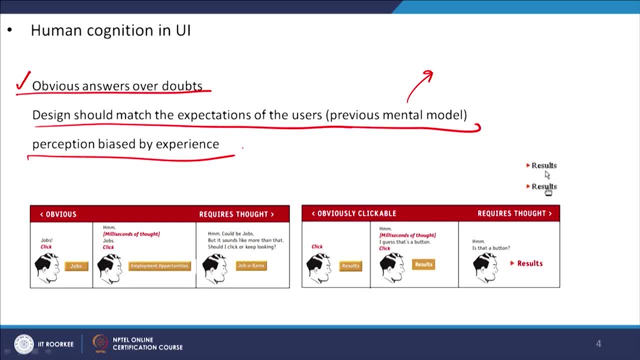 how it will function. So the perception is biased by the user. So the perception is biased by the user. So the perception is biased by the user. So the perception is biased by their previous experience. Their experience changes, and each and every. that is why different user group will have 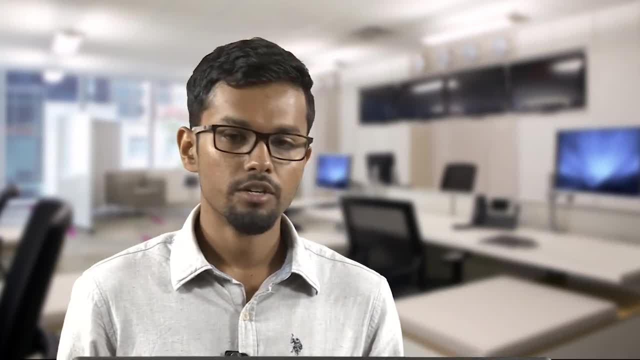 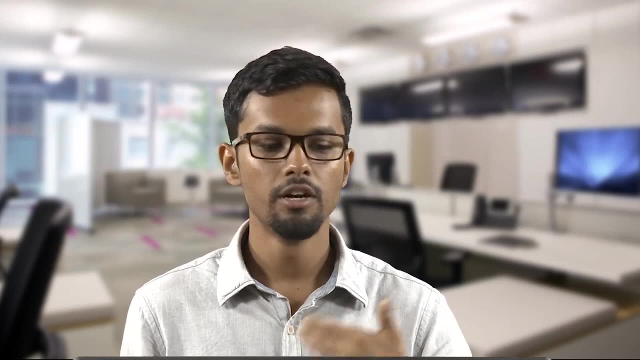 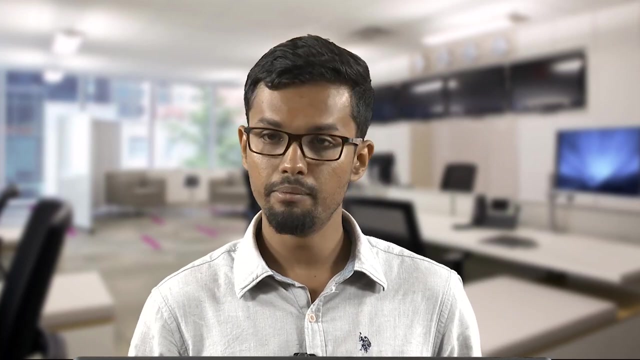 different biases and their expectation might even differ. So that is why identifying the particular user group is the first task for the designers, and then analyzing what will be their behavior will come in the next process. So this is just a simple example from the same book. Don t Make Me Think. 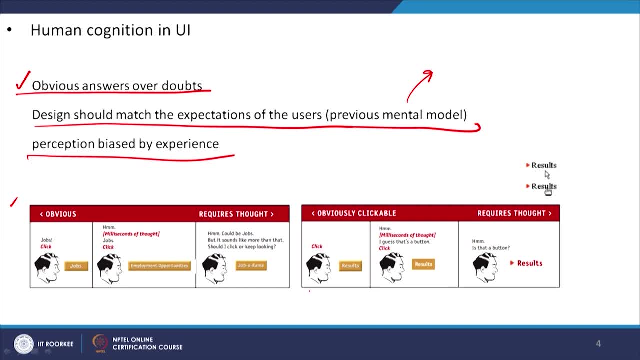 So if we just design and based on just a typology of design and the UI component, how we write what will be the text on the document and the visual communication component, how we are designing the button, based on that, it can be obvious or doubtful. So it can either in this side, this is obvious and this side this is doubtful or requires. 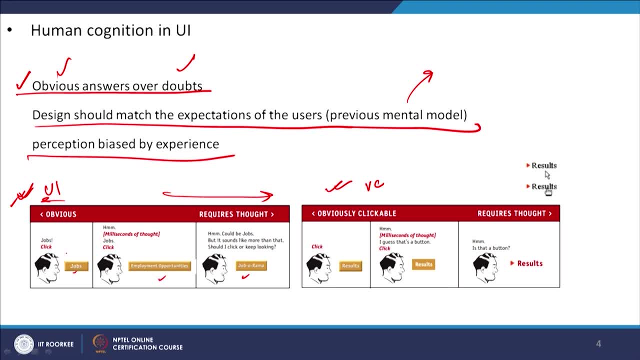 thought: So if we just create companies, HR part of this website, So there is a job options. So if we just write job, that will be more obvious. and then if we write more redundant words like employment opportunity, or we exaggerate the words, so that starts creating a little. 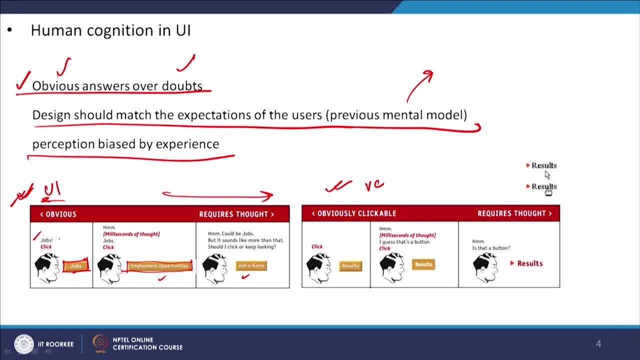 bit confusion. So user will, in the first option they will just think jobs, They will click and they will see different job profiles. Okay, So if we write 2,, 3 more words, then they will start processing and they will start taking more time and then they will arrive to the decision. 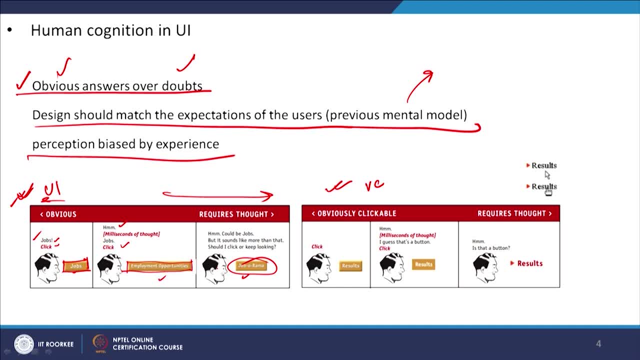 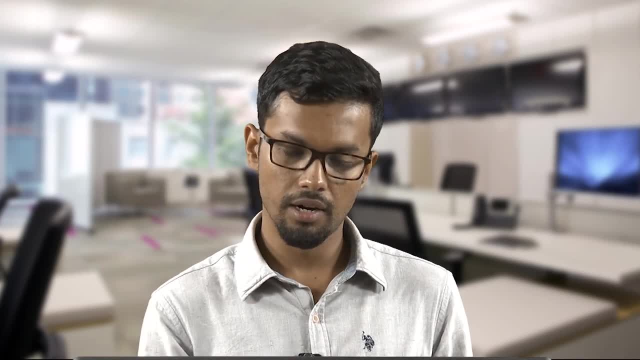 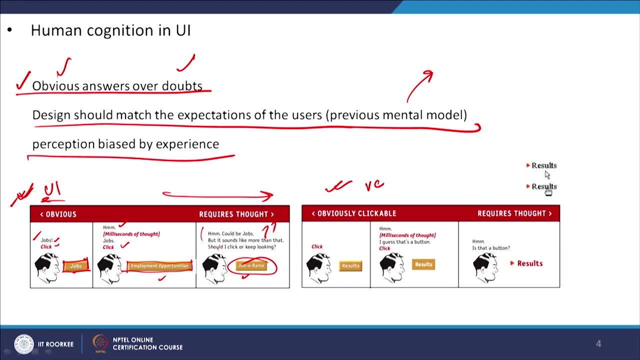 And if we write some obscure words, something which is not so obvious and not so directly connected with the particular terminology, then it will be more and more difficult for the user to interpret, and then they will be confused, and then there will be lot of question marks rather than obvious decision. 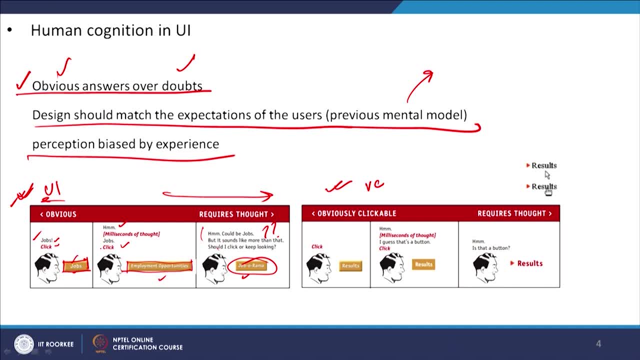 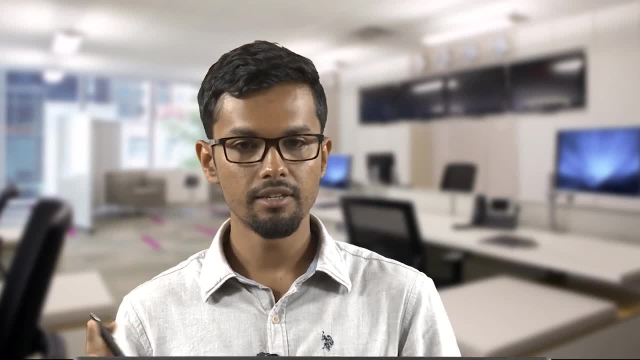 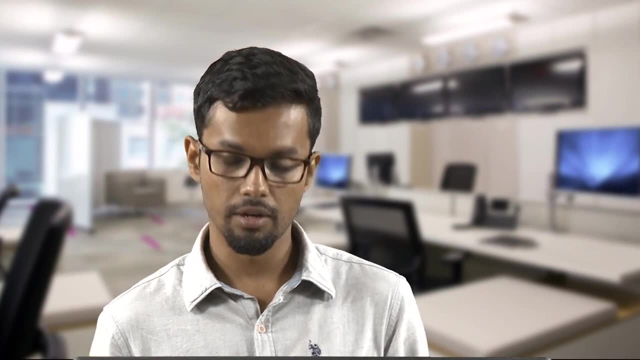 So that was the UI component, what we write in the button. So that comes within the user interface design. and then next, when we are designing the button, what kind of color, whether there will be drop shadow or beveled edge, then that comes a visual communication design component. 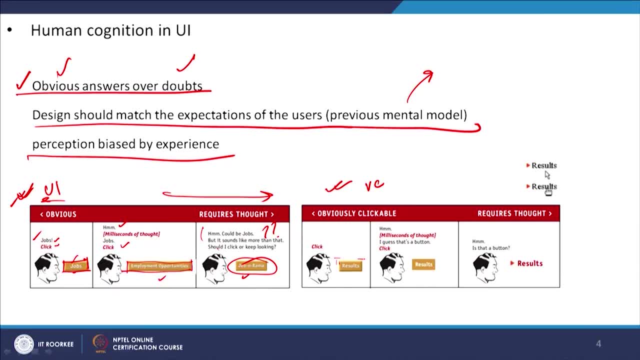 So, for example, if they want a result and the button is like beveled, which looks like a button, So they will click it. So that is more obvious. So if we delete the, if it is like a flat, we are not comparing the material, design or 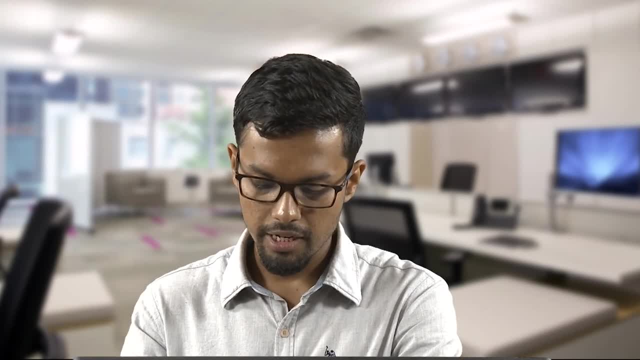 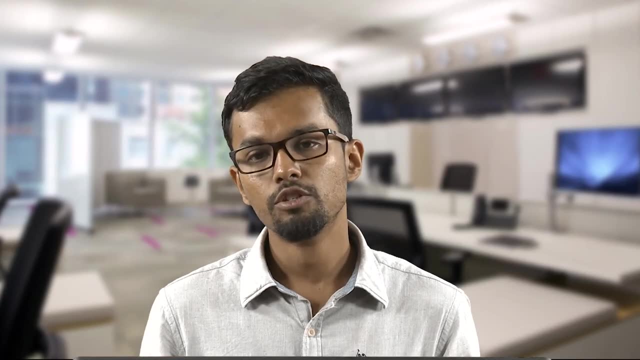 the flat design versus iOS design. So here there can be a drop shadow in terms of material design. So if there is a Google s material design, which we will discuss, what is the visual style? So visual style also differs. There can be a drop shadow so that it looks like it can be clicked. 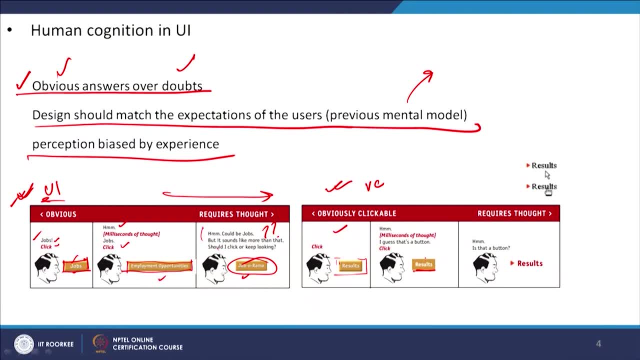 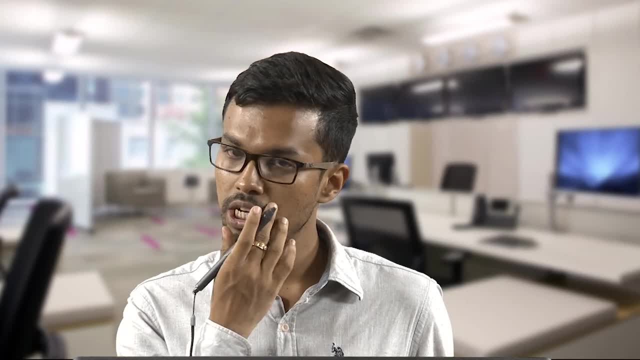 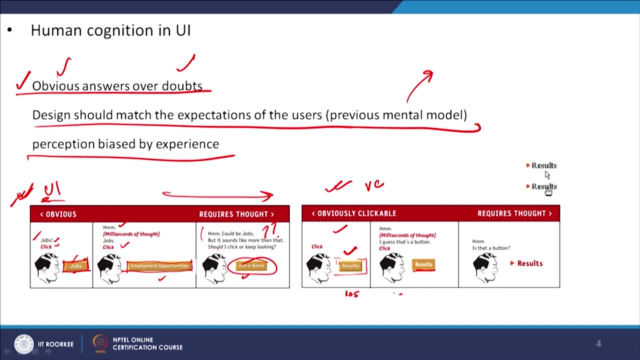 So it is not just whether there will be beveled edge or not. It can even be flat, but if there is a drop shadow or something, some visual cue that this button can be clicked, then also it will be an obvious decision. So it is not a comparison between iOS and material design. no, 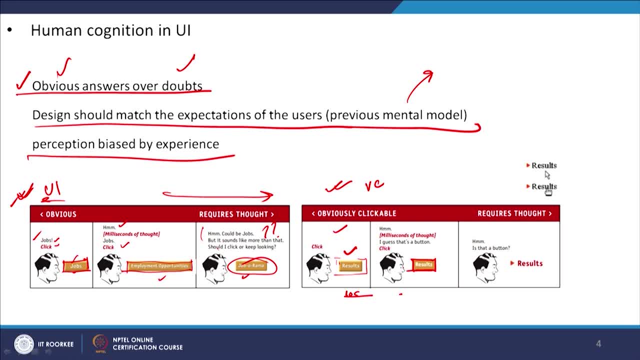 So if the button does not give any visual sensation that it is already clicked or whether it can be clicked- because sometimes when there are multiple buttons, you can also see the buttons are designed like this- So this button, if we look at This button, is clicked. 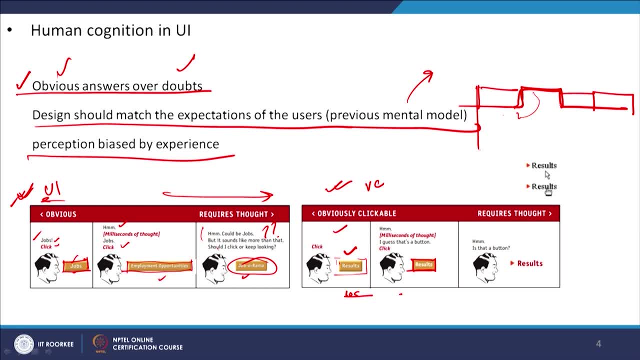 So because this is joined like that, so we cannot click this button again, So we will land on to the same page and these buttons can be clicked. So there are different other ways to treat this. in terms of visual communication design, We can treat it in a different way. 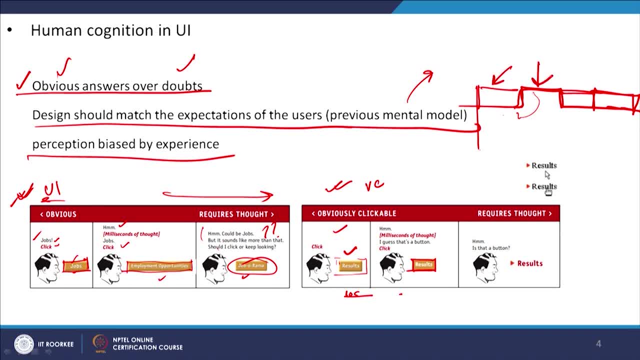 So if we treat it properly, so if there is a difference between these two buttons, so that becomes obvious solution. If there is no difference, so if we design like this and if we do not know which button is clicked, So everything looks same, Then it falls under this: so whether we click it, so they will again click the button and 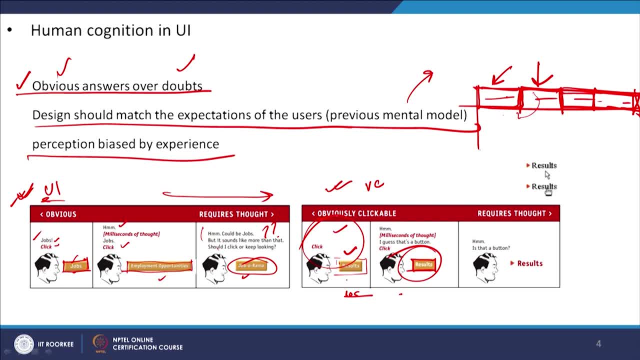 they will become more confused. And if this button does not even look like a button- for example, it is like it looks like a drop down or something- then they will not even understand. So if the only solution, if they by chance mouse over the buttons, the mouse only comes, 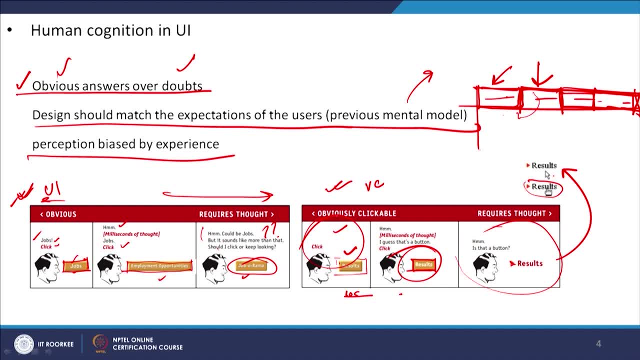 on that, then it can be like a hand and then they can understand whether, okay, we can click it, So otherwise they will be missing this button. So this also creates lot of confusion. So, based on visual communication or UX design component, how you are designing. 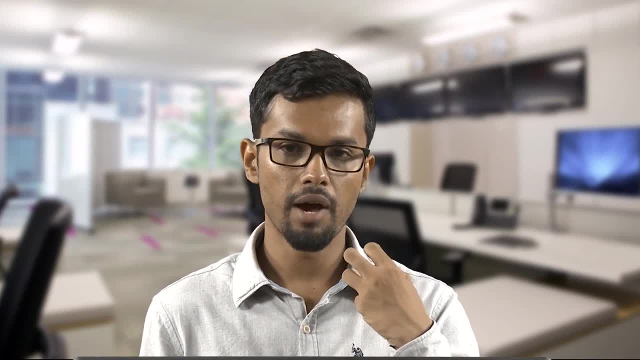 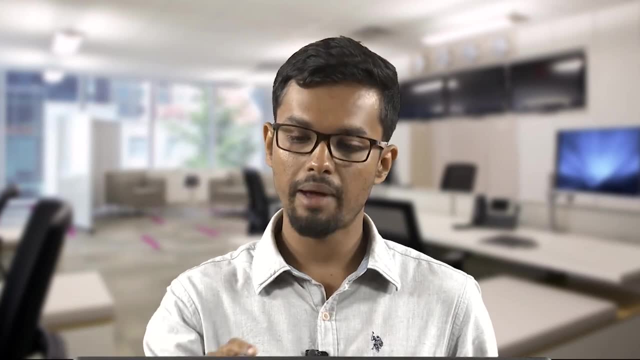 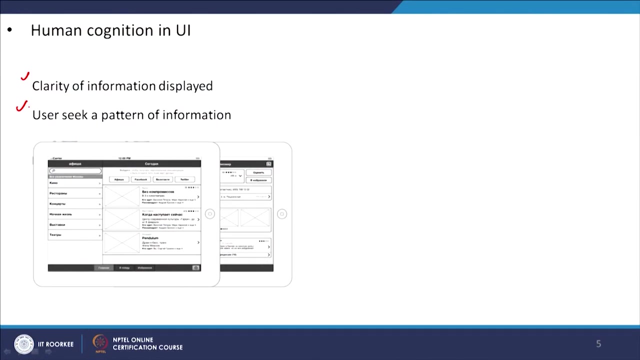 So you always need to think about, you have to provide them the obvious solution and obvious function so that their mental model, their expectation and the function matches. Next is when, many of the times, we have to provide lot of information because I was just telling that their expectation from a particular website. 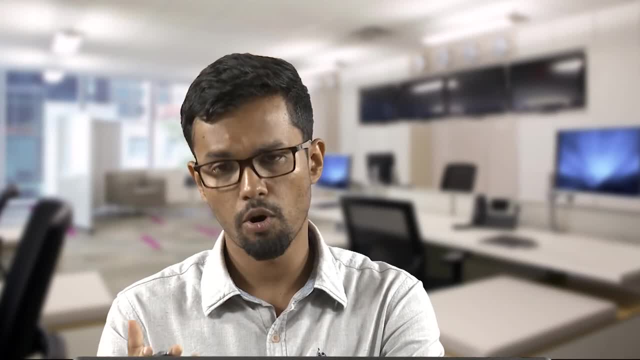 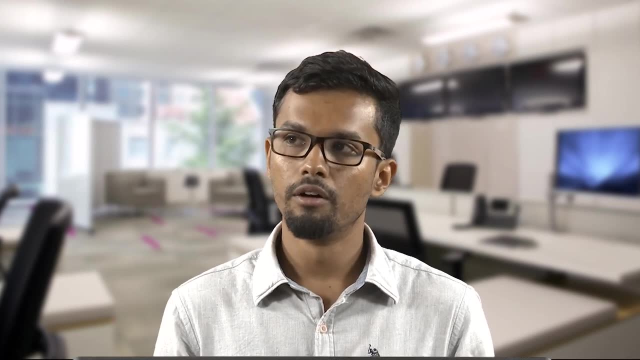 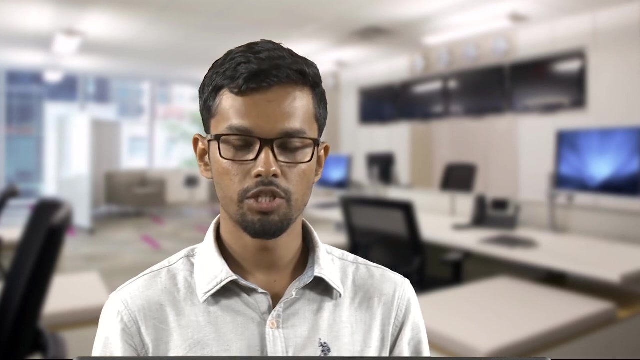 function of a particular website or the product, the expectation will be more, So they will expect the product to function, perform different task. For example, if you see, the first initial mobiles were just to make calls. Now the mobile phone includes watches, includes many things which. 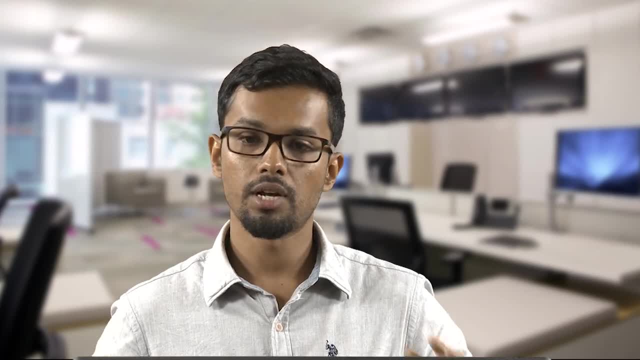 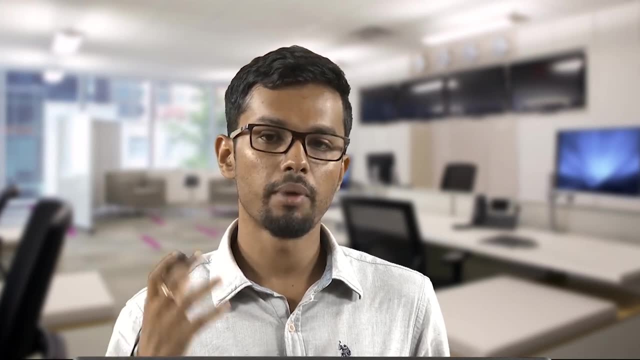 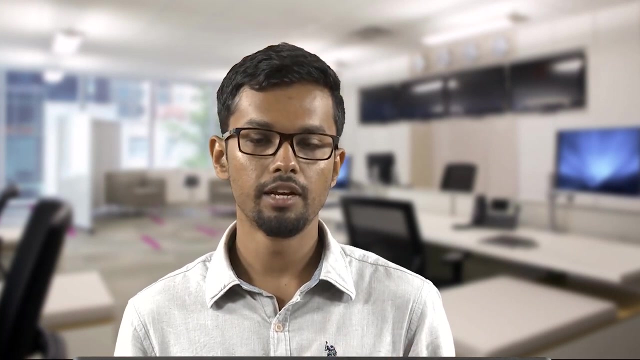 was not envisioned earlier as a performance task of the mobile phone. So they expect- because the user wanted or expected- many tasks to be performed by a small device. That is why this features got added. So they will want lot of task to be performed through a single website, but they will. 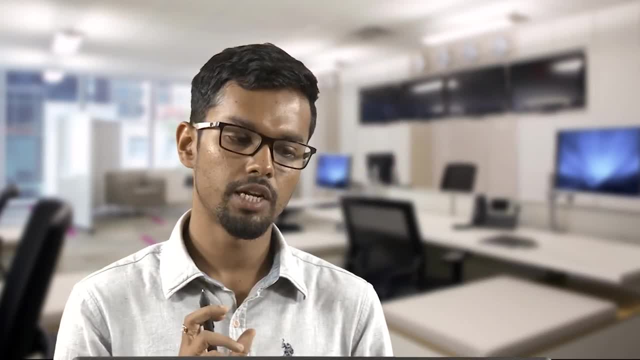 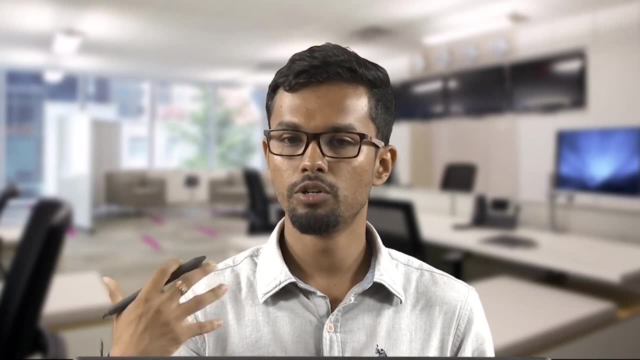 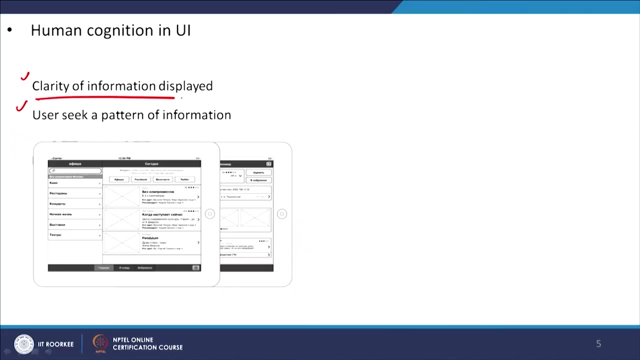 want a very clear and small step for each and every task. So the information, what you need to provide, will be more and more if you want to cater to different task, But when we are showing the information, the clarity of the information, you cannot compare two different стоck like, let us sayiedo, You have to compare two different. 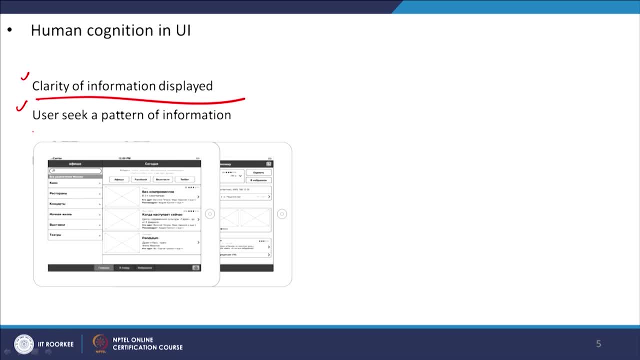 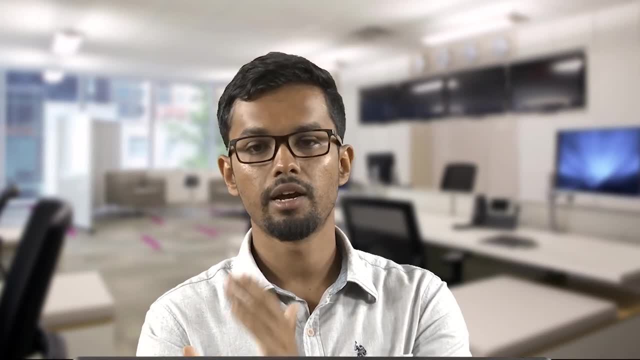 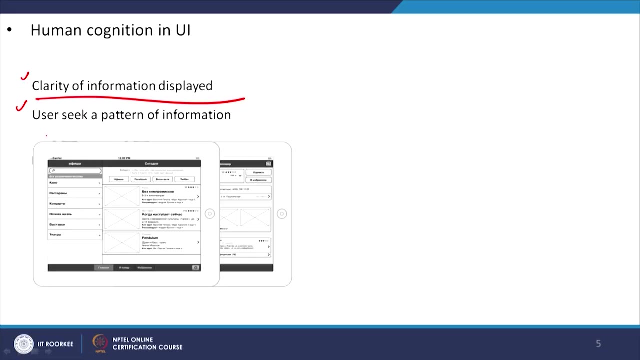 information displayed has to be there. That is the main focus and we will discuss how to achieve clarity and how to do all these things in terms of visual design and universe design when we discuss that particular subject. But what user want from their perspective, is they. 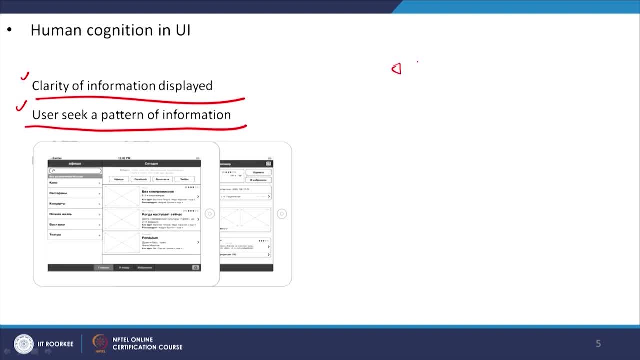 seek a pattern of information. So when there is a different information there, if there is no link within this information, they will be lost within the information. If there is a one type of information are placed in one side. another type of information is another category. 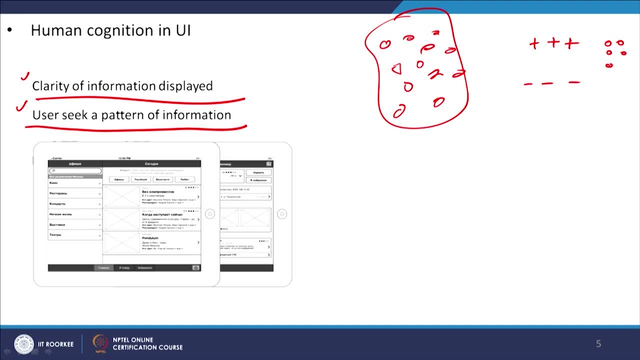 and other type of information are placed in one part of this webpage, then they will understand. okay, this is the type of information here. This is another type of information and this is another type of information. By looking at different option, they can negate what they do. 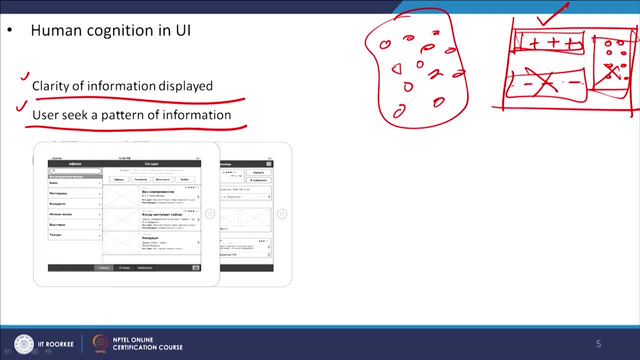 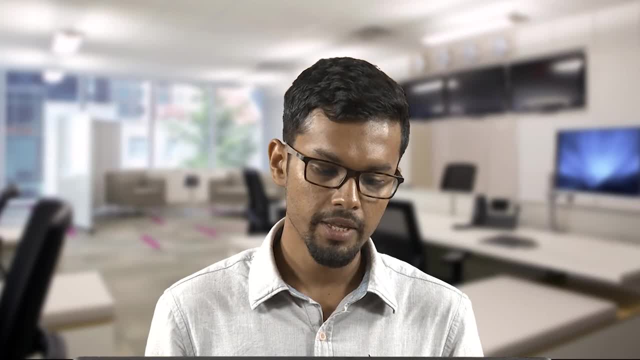 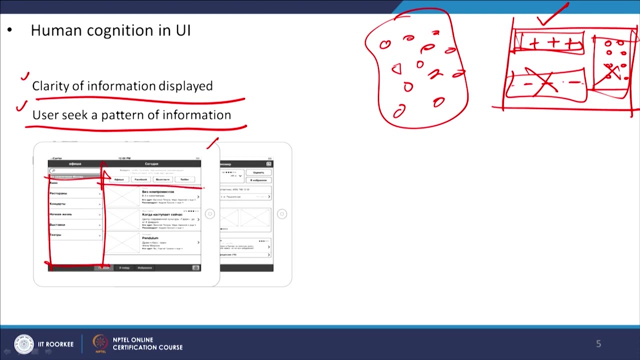 not want and what information they want. So just scattering the information will not work. So there has to be a pattern within the information. So in better design you can see a particular type of information will be clubbed in a particular site and another type. 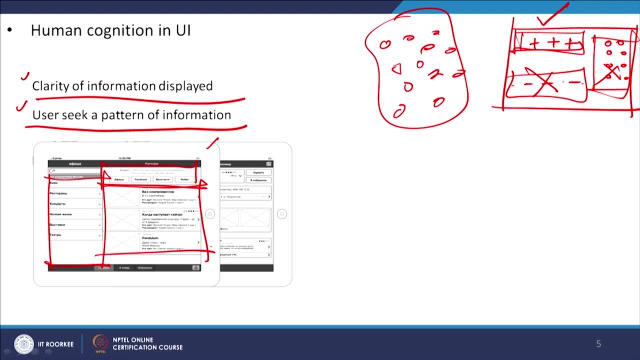 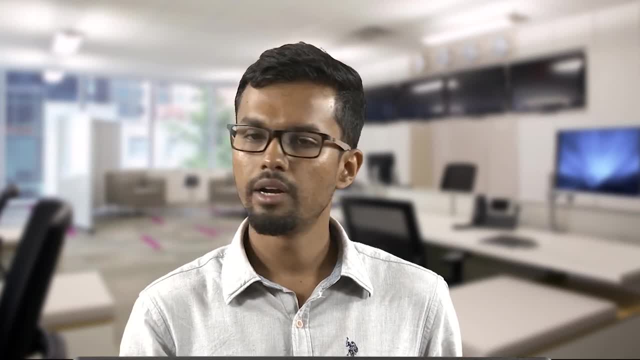 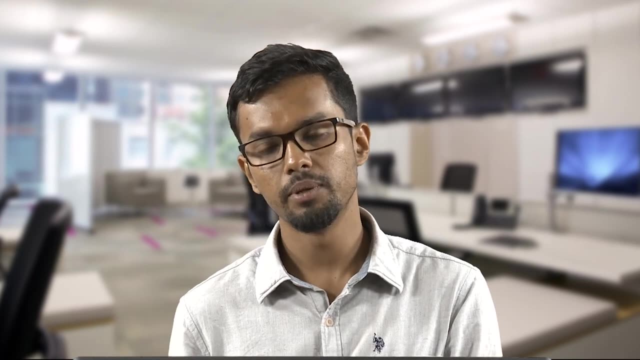 of information, another type of information. So there will be different parts which will give you similar kind of information so that the user can interpret the information in a better way. So there are many other ways to club. So we will discuss gestures, principles and other visual cognitive principles to achieve this and how visual design can help. 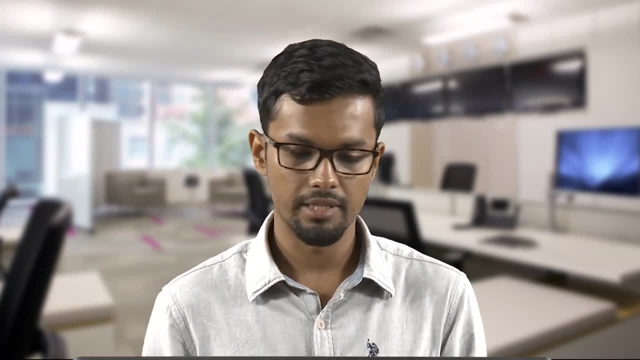 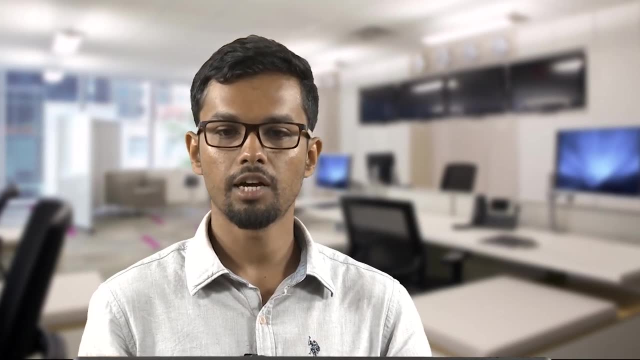 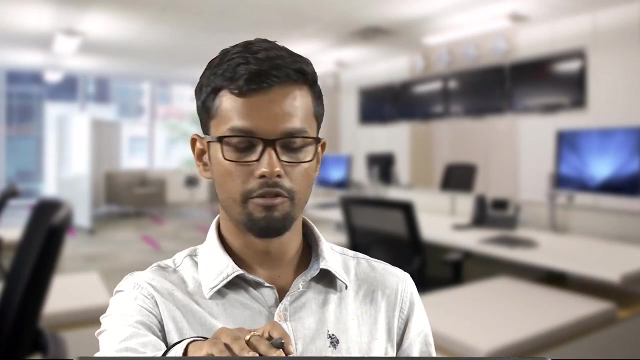 UI, UX design can help in this. We will discuss that. but the thing is the user will. user want a pattern of information, otherwise they will be burdened within the plethora of lot of information. They will not able to perform the task. And within this information also, they want clarity of navigation. So how? 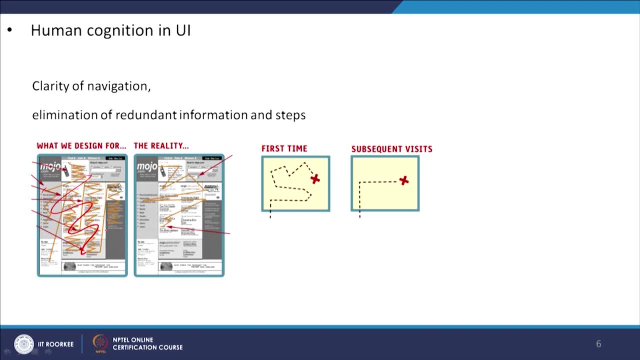 would they know what information they will have and what way they have toizonize it? So how Clarity of navigation is generated. isn't it important to understand about the Toronto Pk Number? do they want to navigate their eye and how do they want to perform the next task? that is also 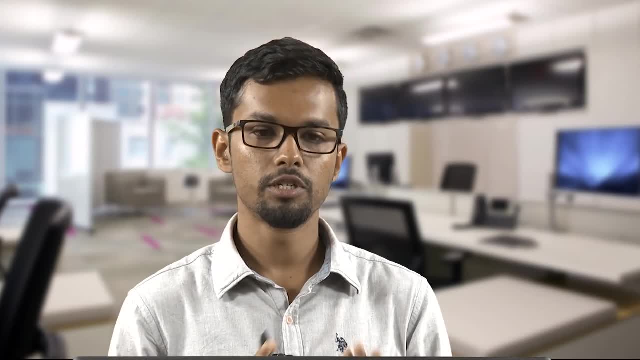 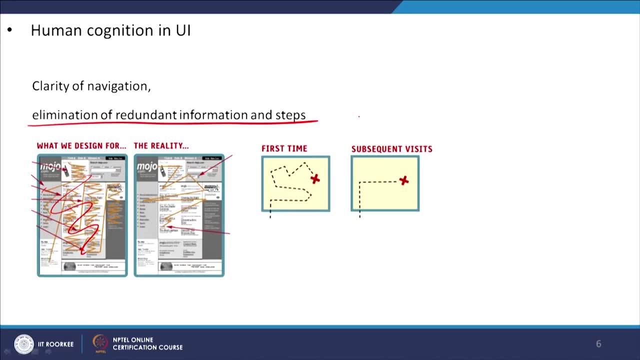 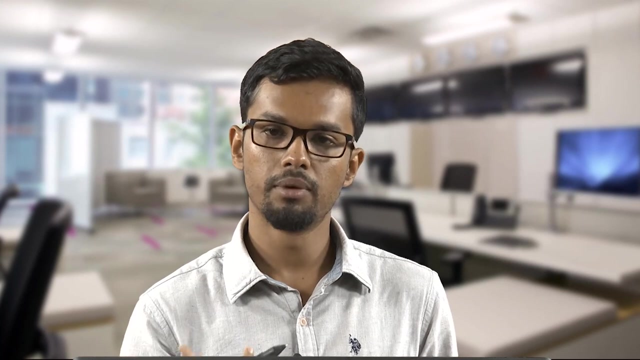 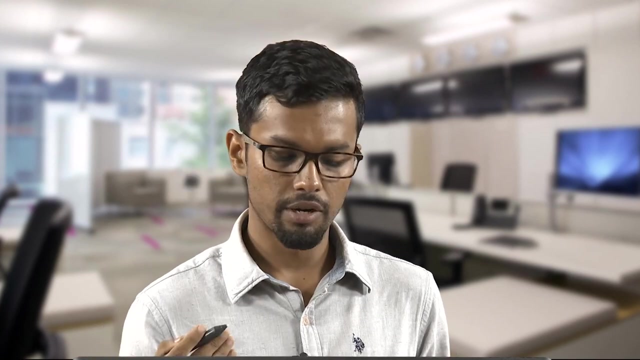 important or also this is clubbed with the clutter of information. More the clutter, difficult for them to navigate within this. So elimination of all redundant information and steps are very, very important. So within that, if the one word can solve and one button can solve, one stage can solve the task, we should definitely look forward for that. 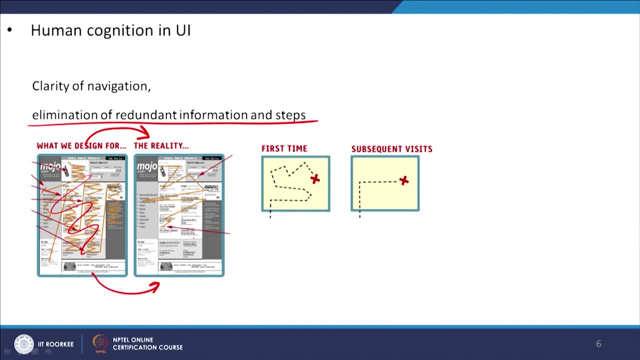 So deletion of data has to be there. So more the data, more their eye will be. They will not read the data. So what it is designed for is to look at all the data, but they will not. They will just look at few data. What they are not looking at, they act. 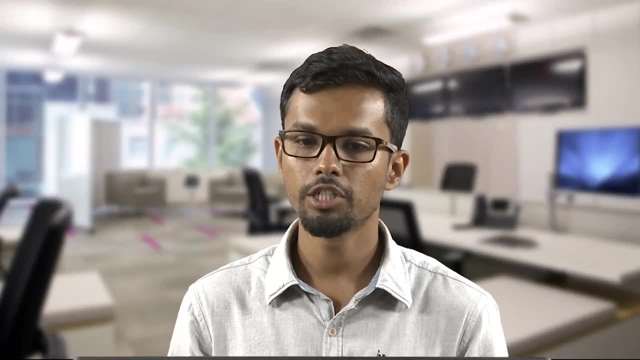 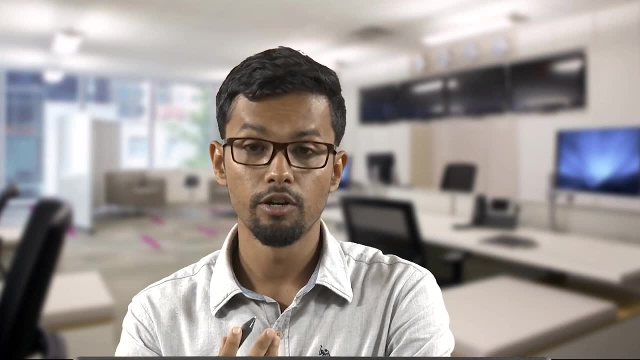 the same way. So there is a difference between two types of information. There is another type of as a redundant information, and that function will not be fulfilled if they are not even looking at it. So there are processes of understanding, where they are looking at, where users are looking at. 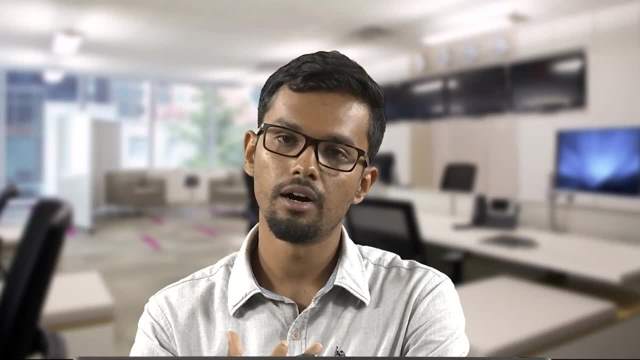 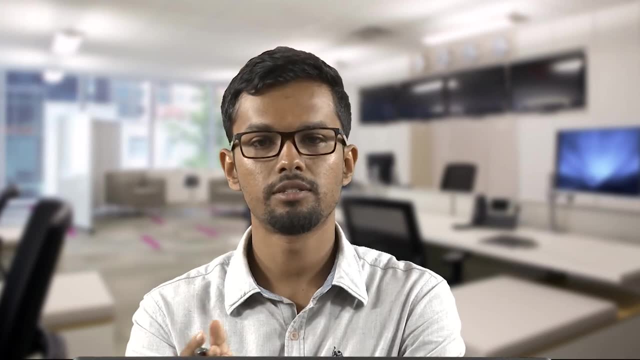 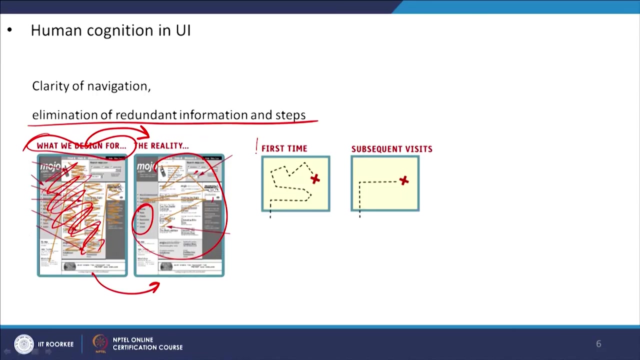 There are theories. Also there are testing, like there are eye tracking process, So users eye can be tracked whether they are looking at a particular site or not. So there are eye trackers, equipments for that. We will show few examples of eye tracker analysis in later classes. So redundancy of 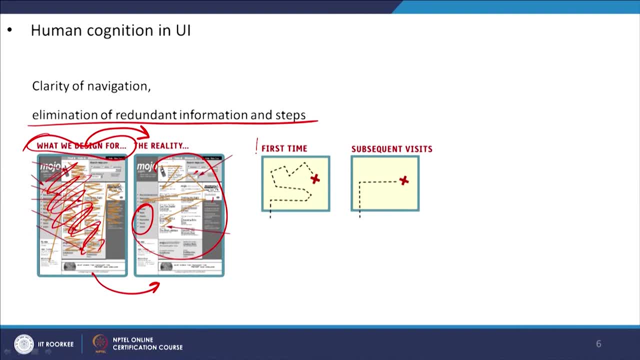 information, more clutter of information creates difficulty, and the stages also. if there are difficult stages, they create difficulties, specially for the first time users. First time users will not know how it will be performed. Subsequent visits can give you a better performance, but if these two matches, if the first time and users. 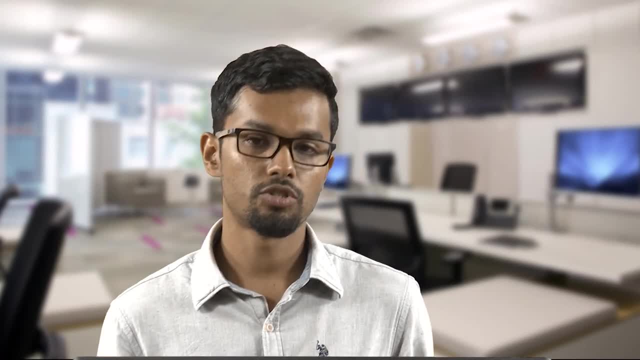 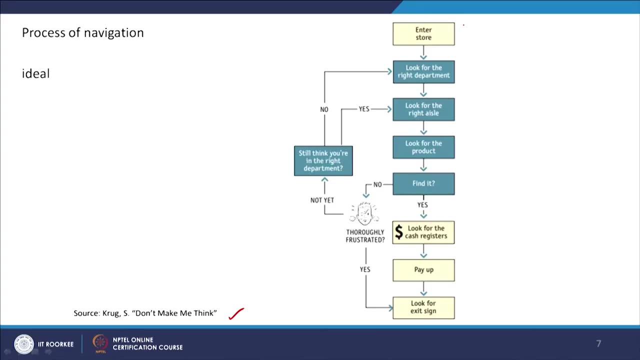 would have to account for the third time and ultimately also 관심 episode. do not give theyYa perform like a subsequent visitors. then that is the best solution. So their expectation exactly matches with what they are looking for. So this is from the same book. Don t Make Me Think. 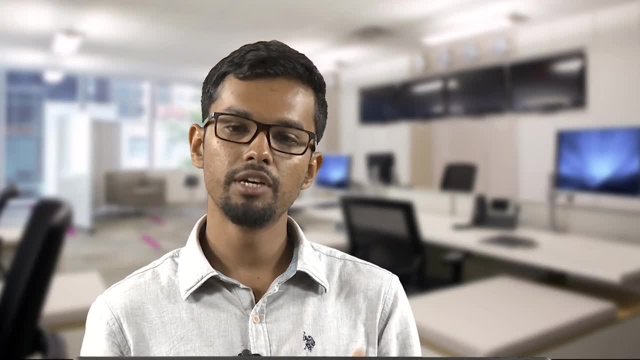 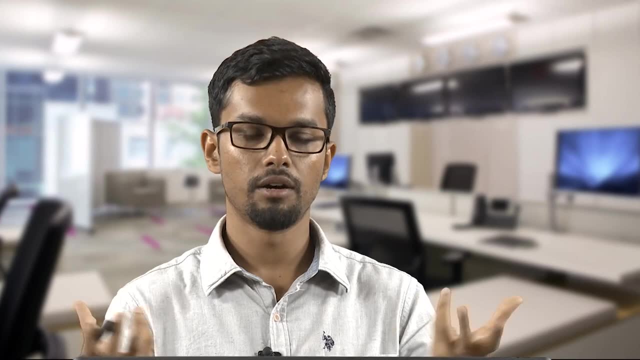 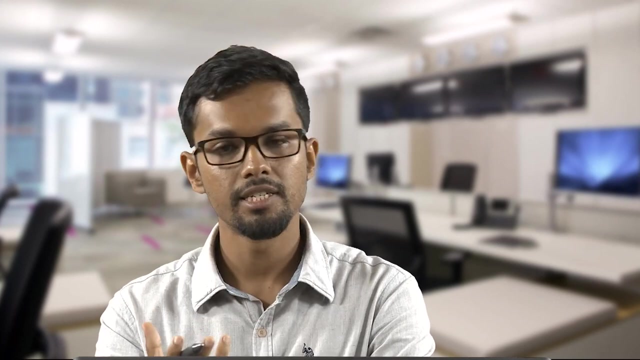 So this can be compared. So this process of navigation in UI, UX, can be compared with the navigation within a space in architecture. So within that around us we have lot of buildings, informations, navigational signages, Through that we can navigate within a space. So, similarly, 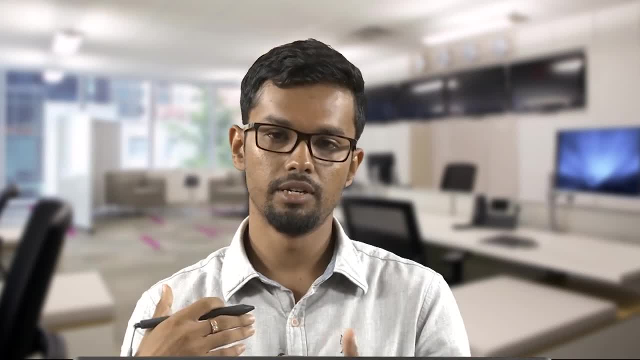 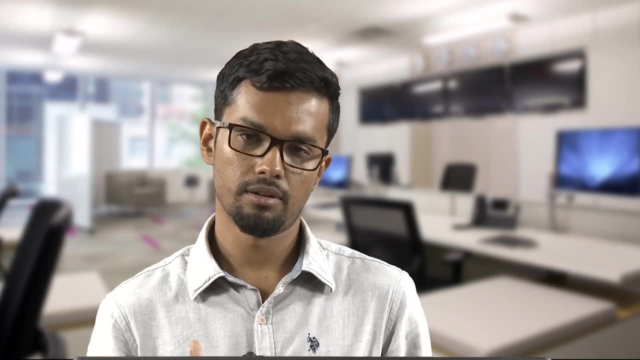 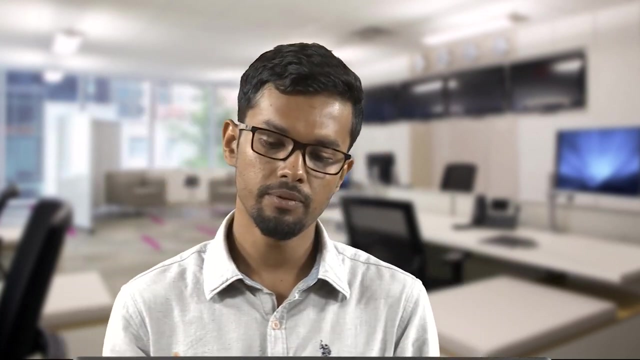 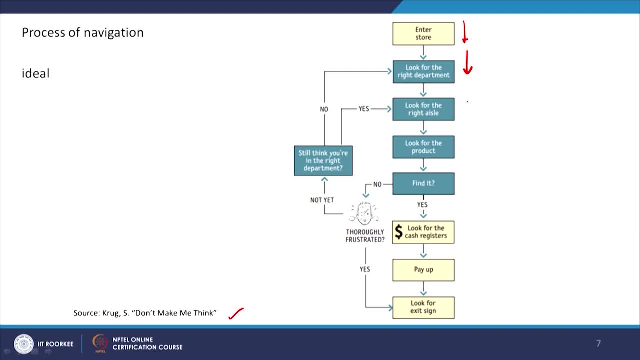 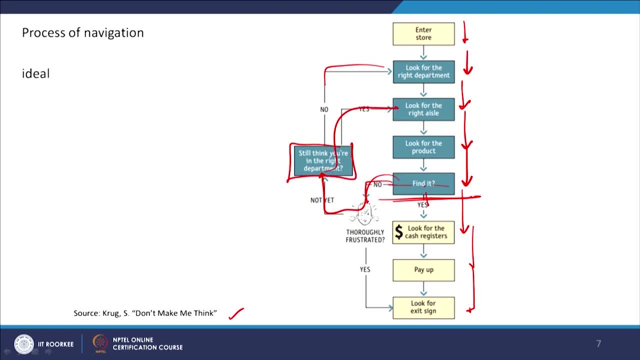 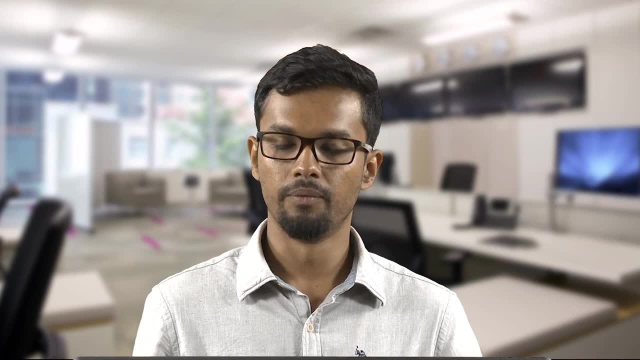 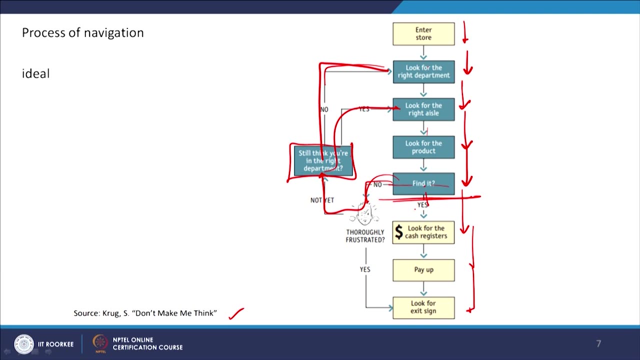 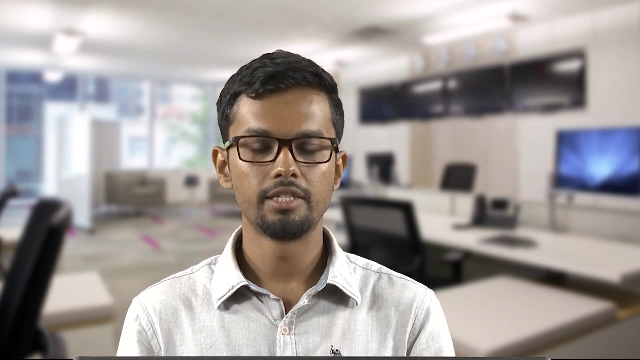 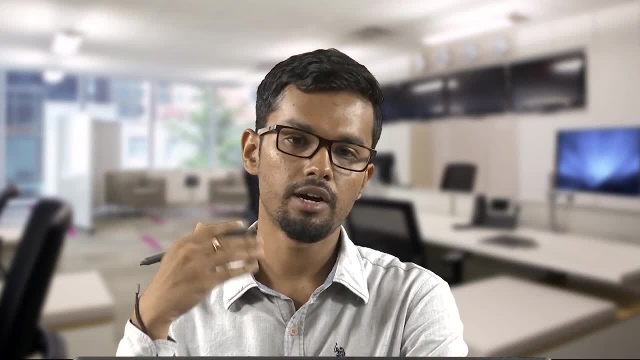 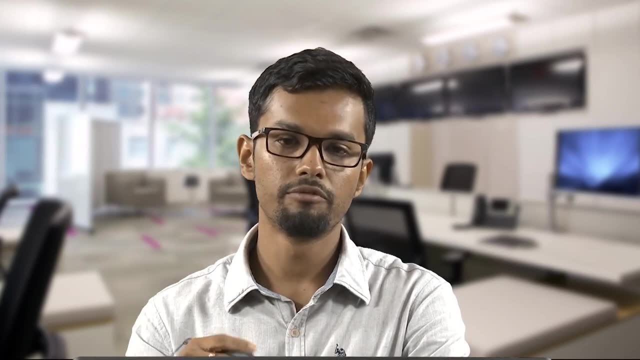 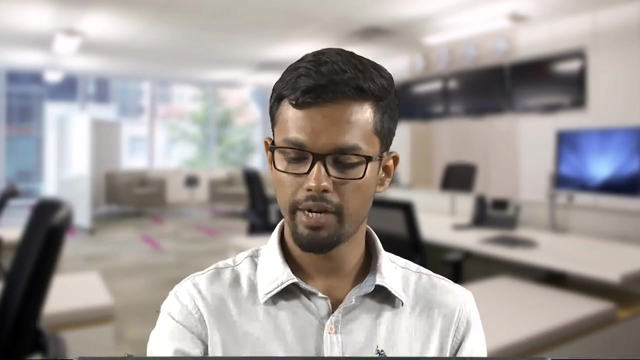 different typology of products and then we start going to the next level, of interfaces. So if we do not find that, we will again go back. So if the interfaces, if the design is proper, this will be a straight line and it will be the quickest process. 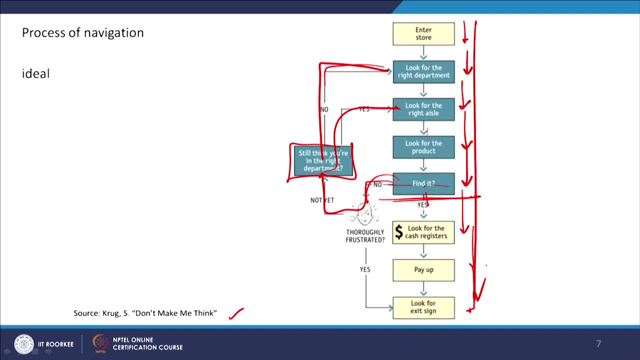 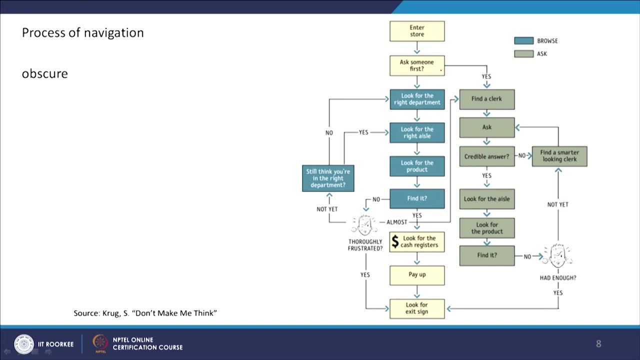 So if the interaction design is designed logically and the steps are very easy to perform and it puts lesser cognitive load on the user, it will be like this and otherwise there will be lot of confusion. Now, within the store, there is a helper to help people, but within this interface design, 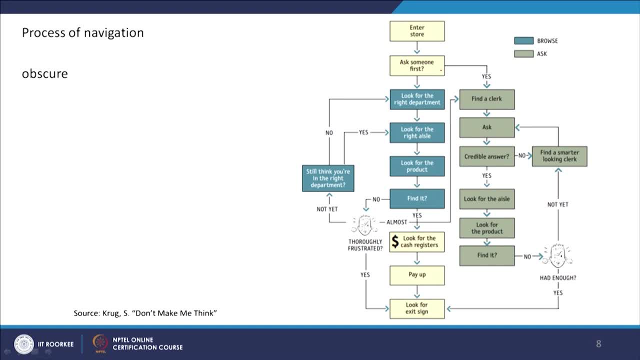 there would not be anybody to help the users. So that is why, within this store- this is again the example of a store- if they have a probability to ask people and then they can always cross check, But within this e-commerce platform, This website and the most of the web pages, there will not be anybody to assist them. 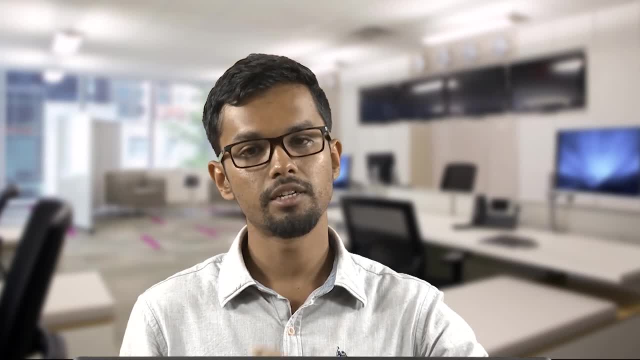 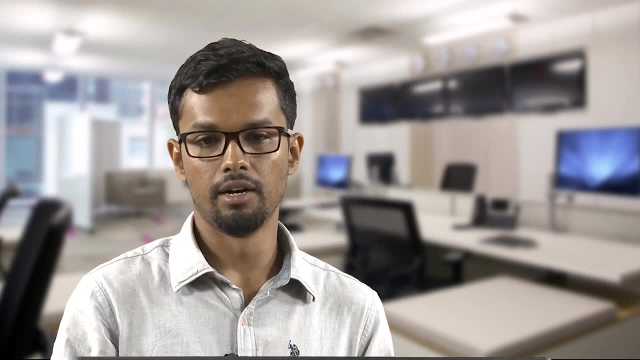 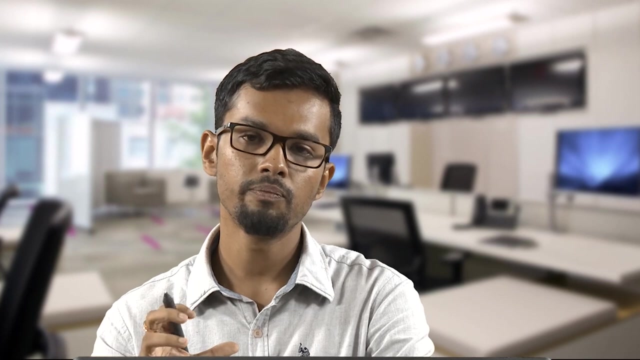 So they will be. if the design is very complicated and not, the clarity is not there, the obvious options are not there and it is not performing the way they are expecting, it is not matching their mental model, then they will be puzzled within the website. 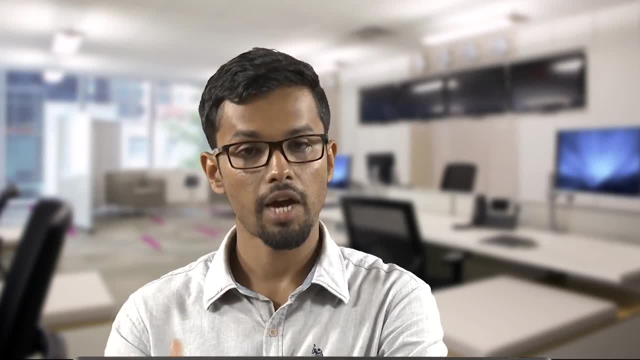 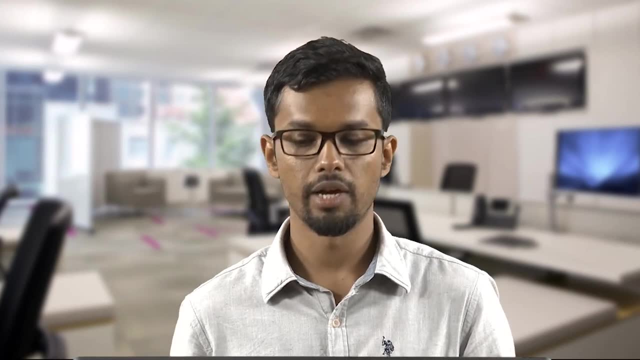 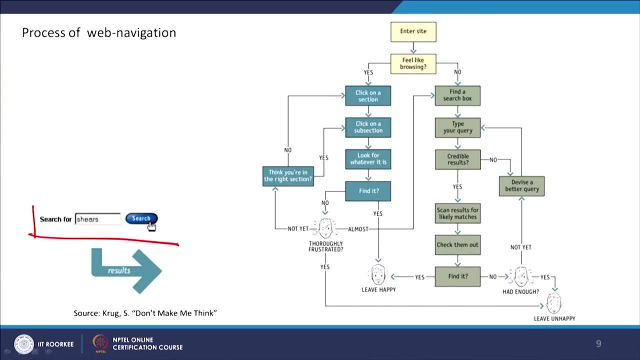 So chances of getting puzzled within a website is much, much higher If there is a, And they will be not be able to solve their problem because there wont. there is nobody to help them. So this is how it has been designed. So that is why there is also a search button which gives the where this particular terminology. 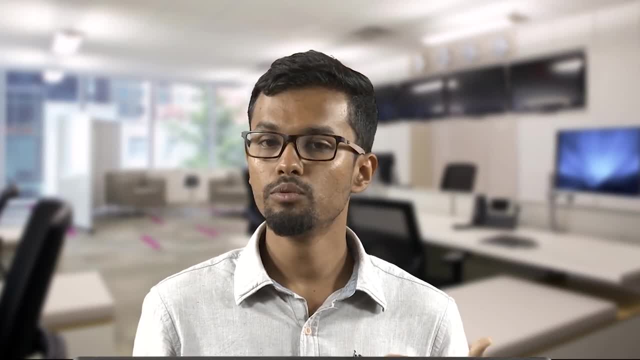 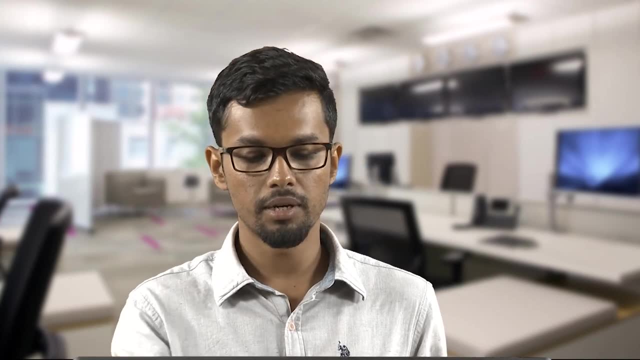 or what you are looking for is there, But search more. they use this search button so this is not a good website. So if the website perform without the search button, it will be a better design. So if all the time they have to go type something on the search, 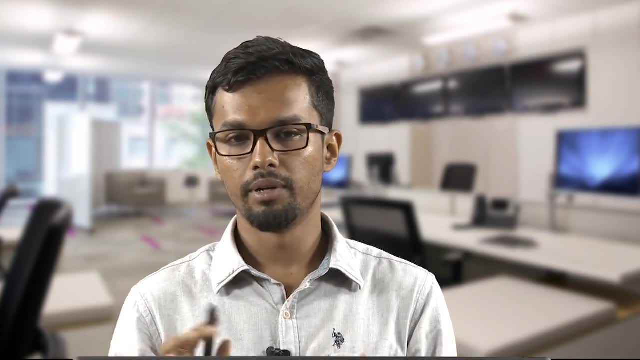 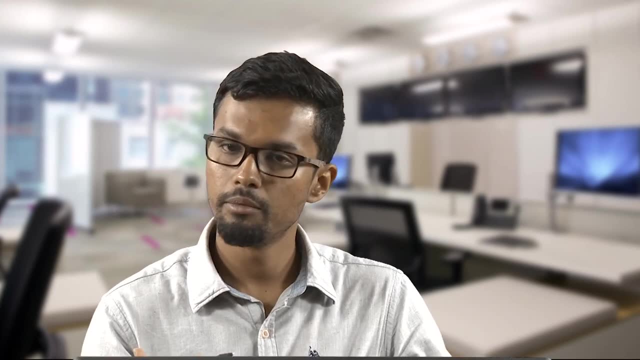 button to identify where exactly they are. this option is so that the website is not performing well. So I am not talking about the search button of ecommerce website, because in ecommerce website we search the product, So that is a essential part of the search button or the flight search. 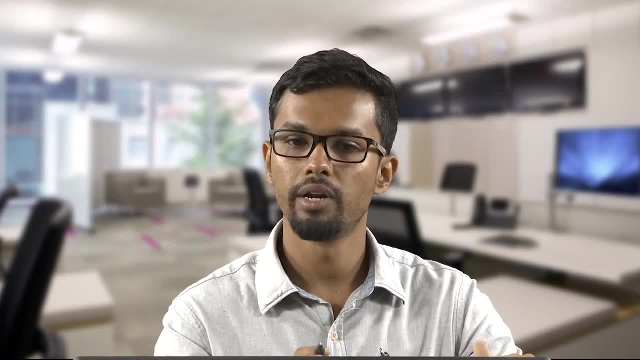 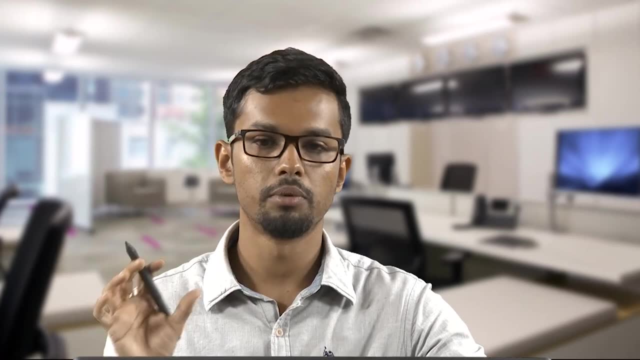 So these are the websites- different kind of websites, when the search button has to be there and which the performance of the search button is different, and will also discuss the position of the search button in that case. So they want the people to search Otherwise in terms of other 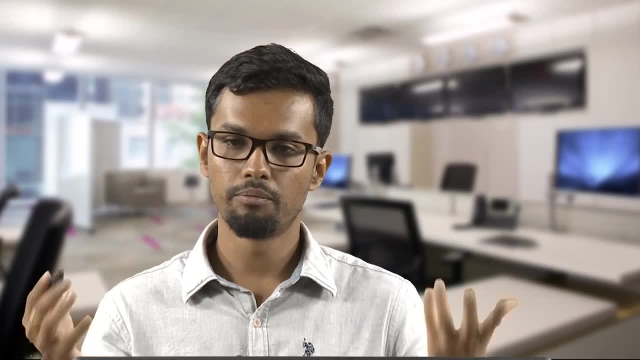 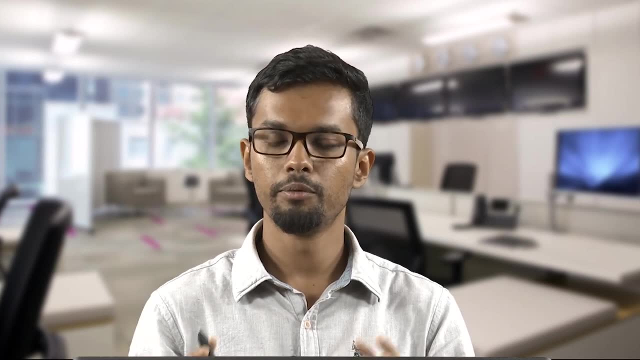 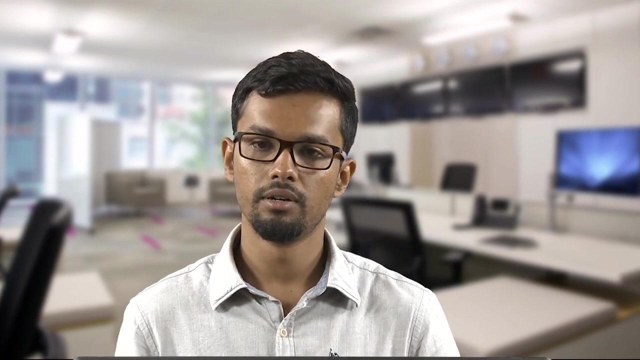 websites, for example, institutes profile page or the website of a particular institute or website of a any company. So there, people should not go for the search button to identify whether there is a job profile or search a particular domain of the website. So they are going to. 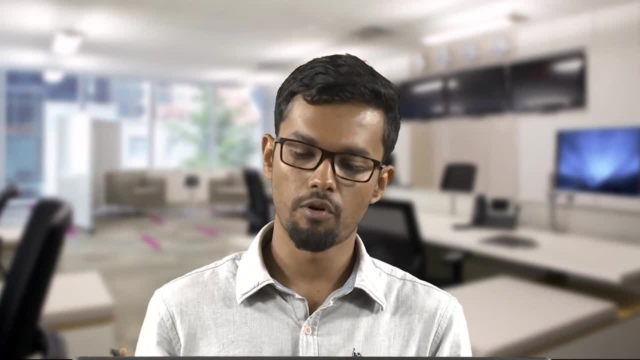 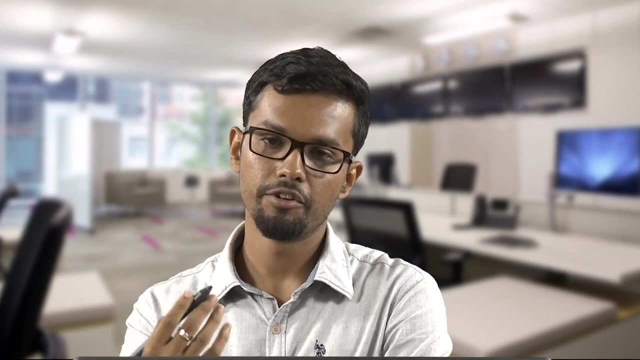 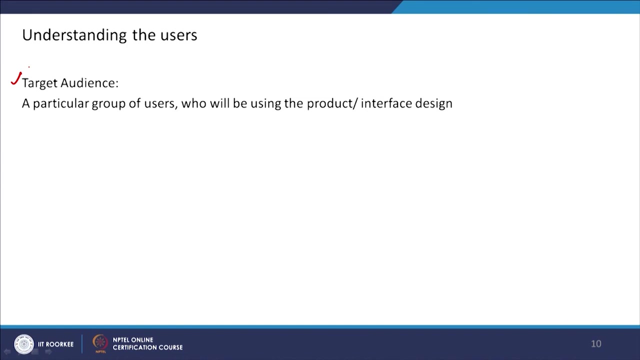 a particular hierarchy within this information page, So the webpage should be self sufficient to help users to navigate within the page. So to identify, when we are discussing about the user s behavior, their common tricks, the important part is identifying the real user, So this is called the target audience In the next class we will start discussing about after. 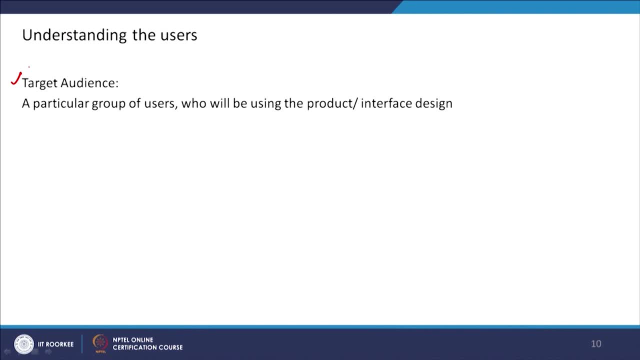 identification, how we exactly pinpoint who are the user, how we find out what is their behavior and how will they perform. But in today s class we will end with the discussion of who is the customer. So they are called target audience, A particular group of user who will be using. 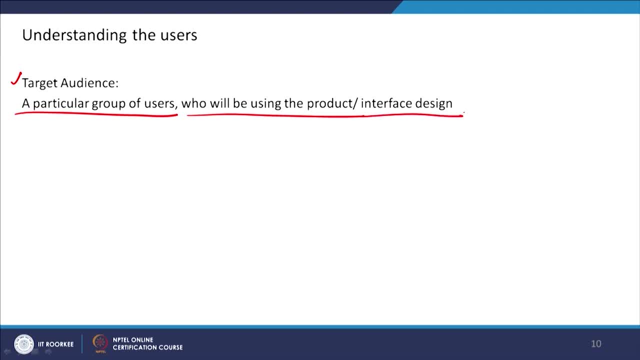 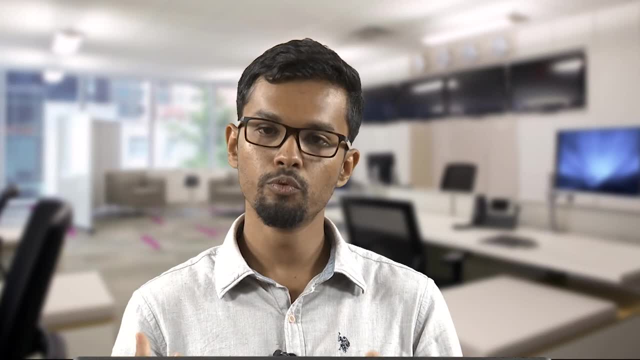 the product. in terms of interface design. it can also be called target audience. It can also be an interface or tangible product, So that group of users are called the target audience, So for whom we are designing, designing the website or designing the any interface. 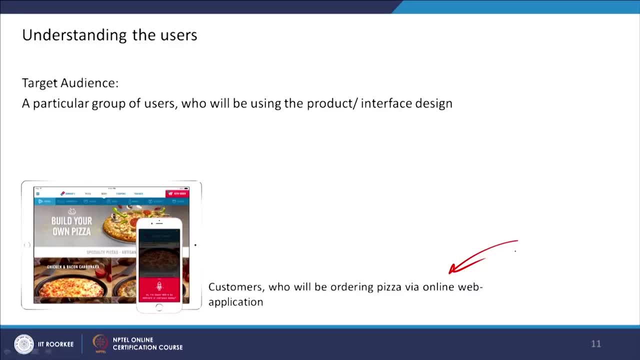 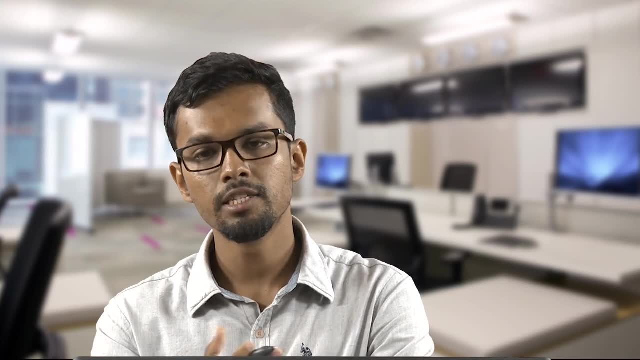 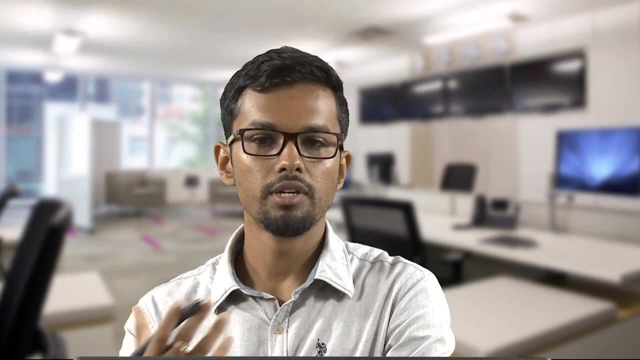 So if we give an example, it can be very defined target audience or it can be even for all. So that depends on the company or what kind of website it is. For example, if it is IRCTC, target audience is huge. So most of the Indians will use IRCTC. 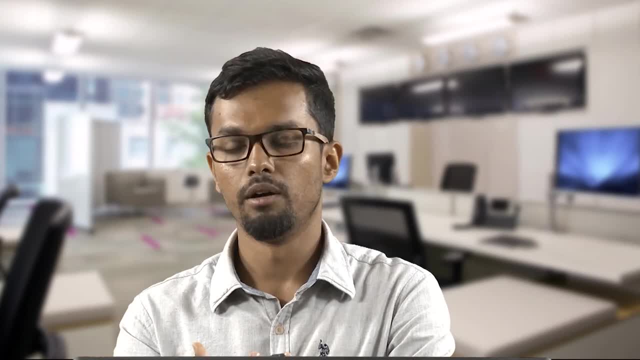 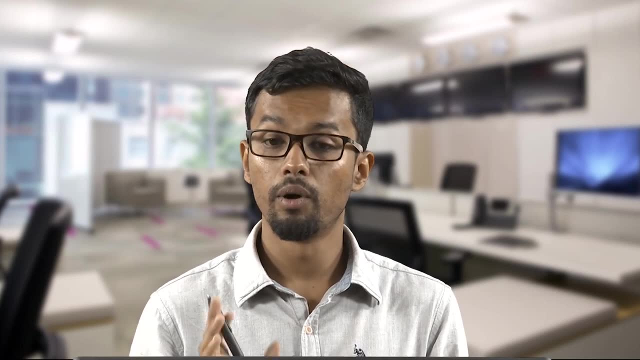 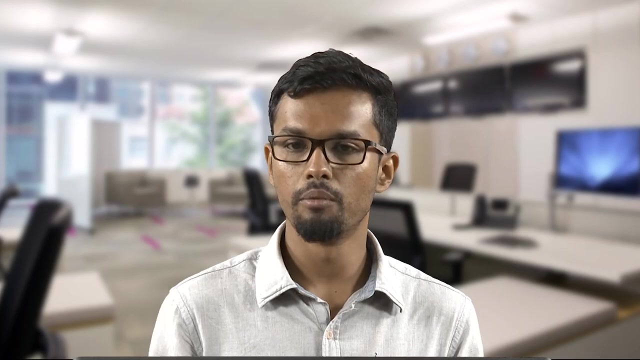 Okay, Okay, So most of the Indians will. who travels through train in one particular certain time? most of us have traveled through train, and this is the only website, One of the most commonly used website. they are competitors, but IRCTC s target audience is much more if we compare with that of a Domino. 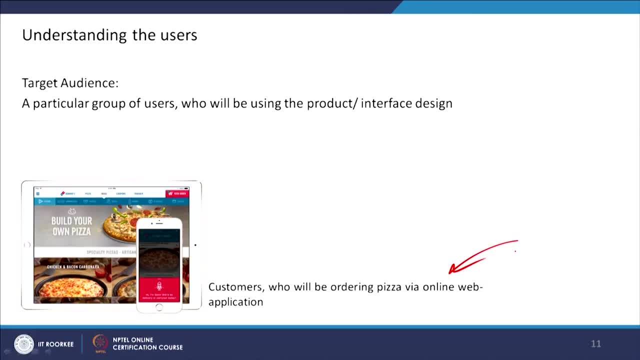 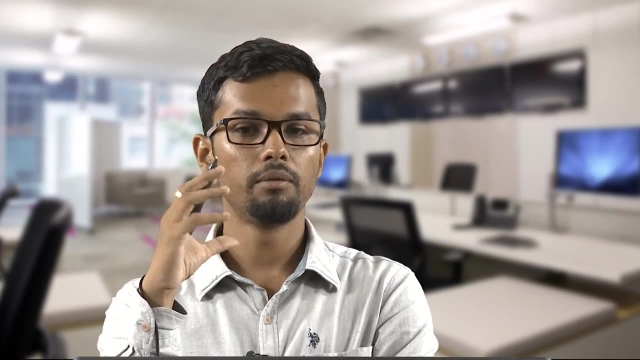 s website users. So Domino s target audience will be only the customer who is ordering pizza via online web application. So that defines the particular users, being Okay. So Domino s has much more defined set of users. So they have a particular behavior And instead. 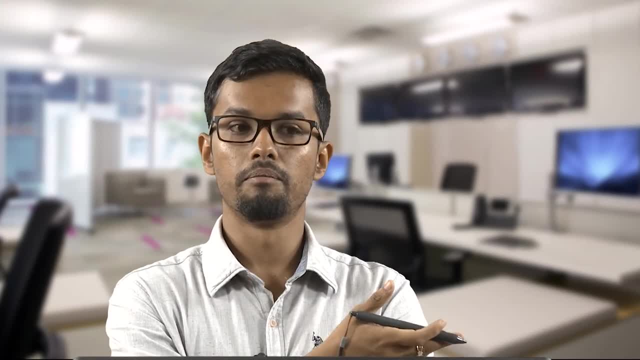 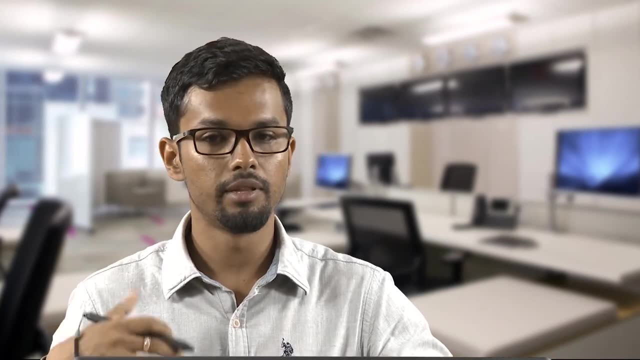 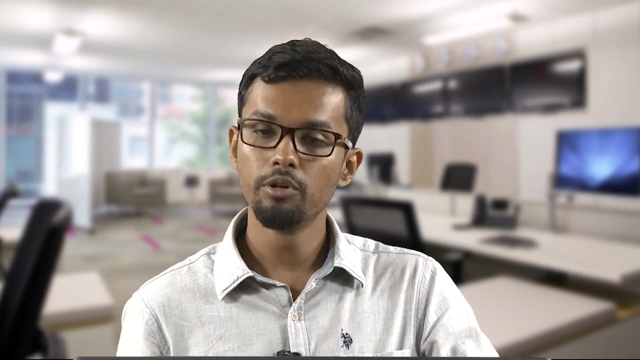 of IRCTC. they have vast range of people to cater So their behavior will change. So different kind of they will have different kind of expectations and their will be more uncertain into the behavior. But Domino s has a very few particular target audience who will be? 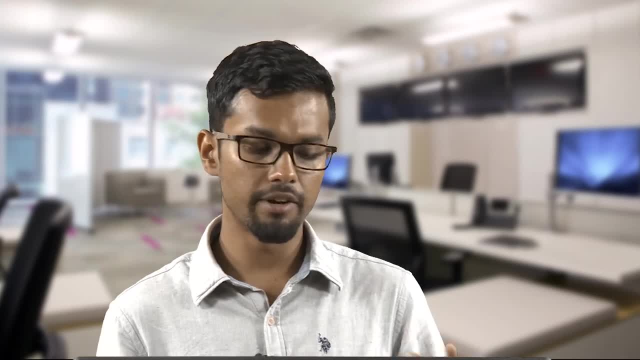 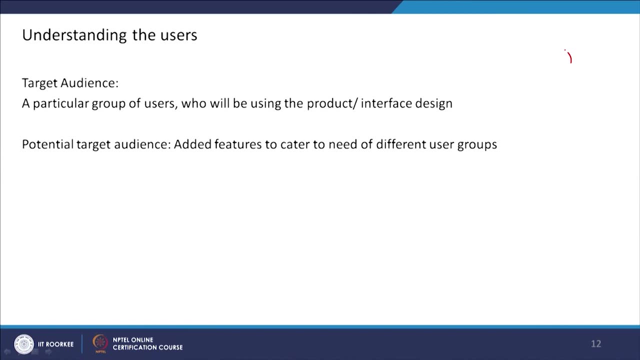 ordering pizza online. So their set s very significant, Okay, Okay, So, certainly Okay. So, in giving other communication and Vetgiving practices as well as writing. so what is the is very, very defined, So that will differ based on the type of company and what we are designing for. 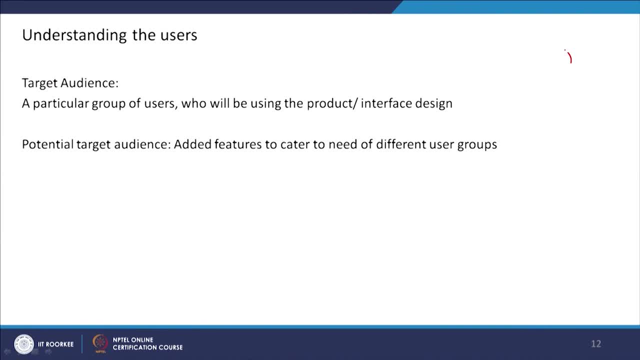 Now there can be a potential target audience, So they are not the exact target audience. but if we change our product they can be within our target audience. If I give an example of a car, so when this nano car was developed, so existing target audience of the car user were not exactly. 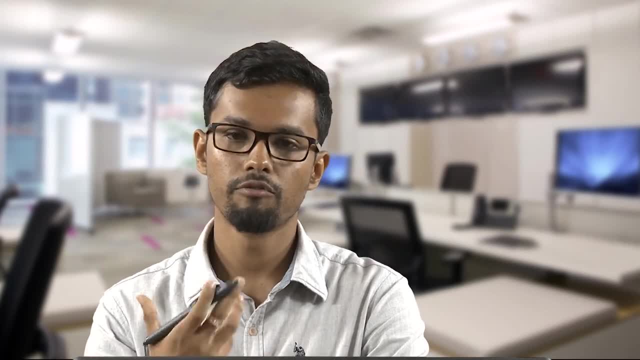 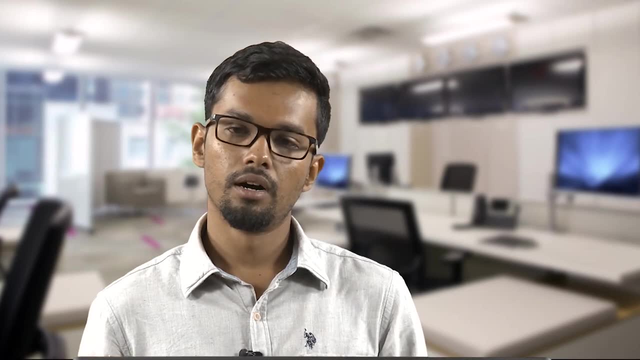 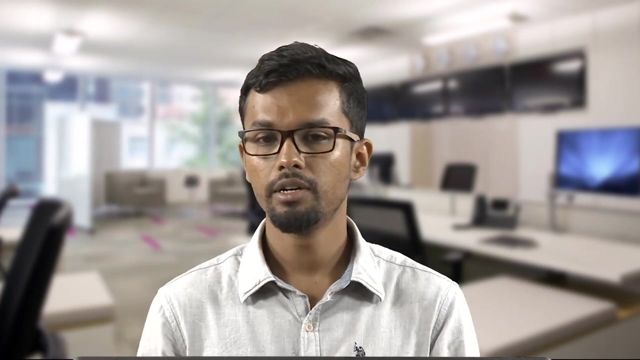 the target audience of the Tata nano car because they were looking for a very low cost car and they wanted to target the two wheeler users, but not exactly a two wheeler users, because their expectation will also be different. Two wheelers- the performance of two wheelers- are different. 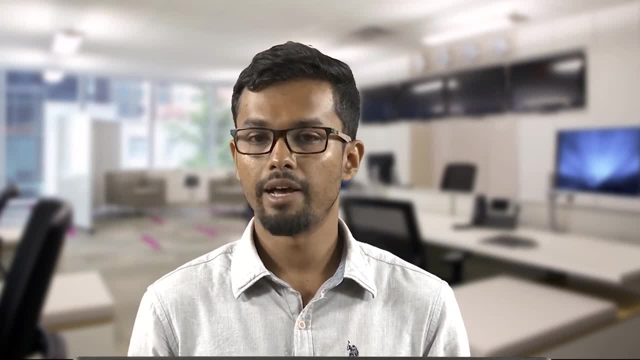 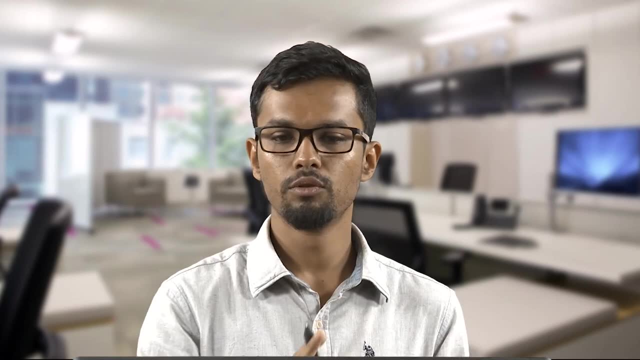 They are not exactly the target audience of the Tata nano car. so when this nano car was developed, the choices some people might be fascinated about, the two wheeler driving, So this is different. So there was something in between the target audience, between the two wheeler users and the 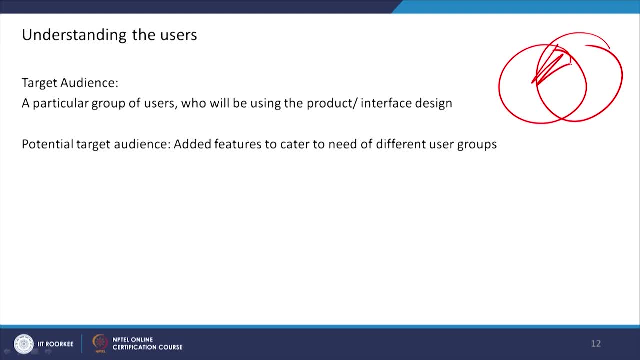 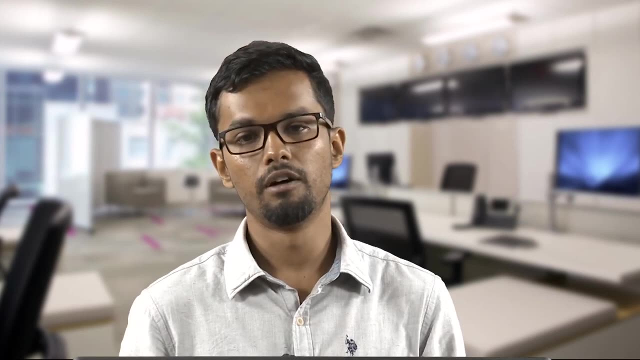 four wheeler users. So there it will overlap. So it might be nano might be somewhere here. So the target audience might not be the- again somebody who will be a potential target audience- who have never used that particular product, Even for the iPad, when Apple first launched. 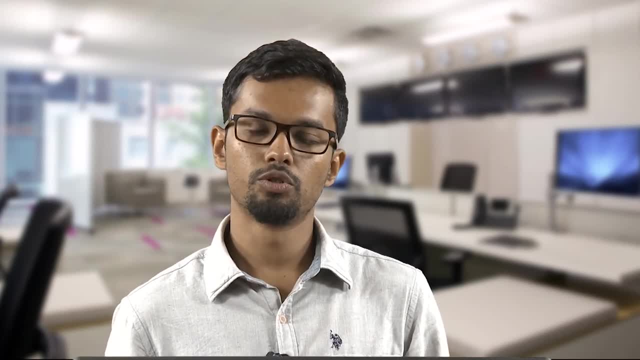 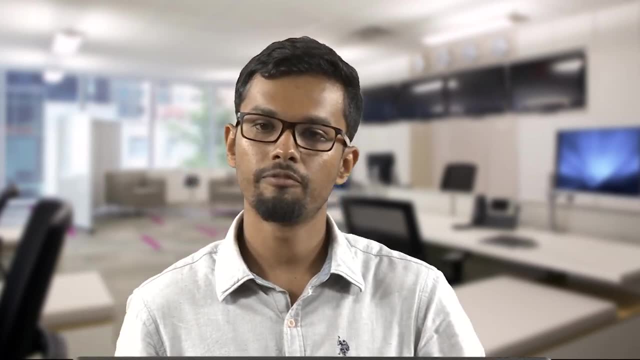 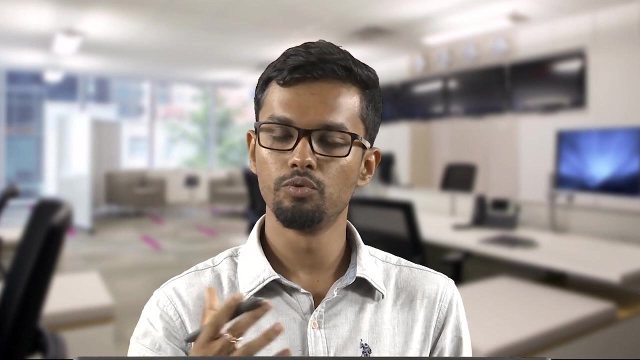 the iPad. it was not even there in the market, So identifying a particular target audience based on existing product is difficult in that case. So, and even in the case of when the product is adding some new features to cater to different type of users, which they are not right now. 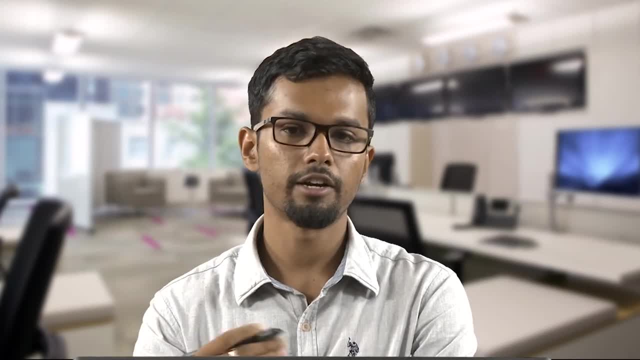 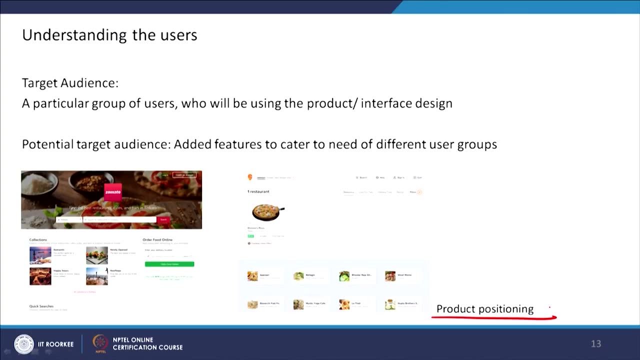 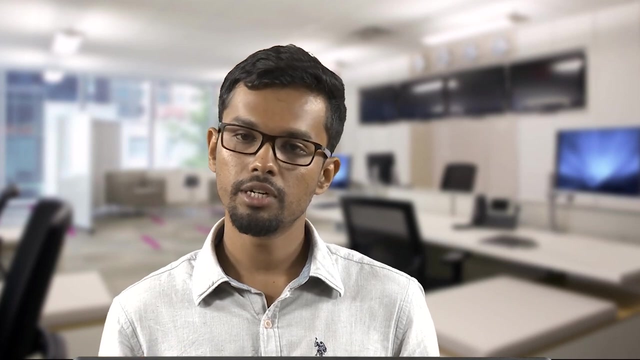 catering to. So identifying them so who can be a potential target audience, might be a different task. So that is also based on the product positioning, how we are positioning the product, So how the same kind of product or same kind of websites can be positioned in a different way so that their target audience also might shift. For 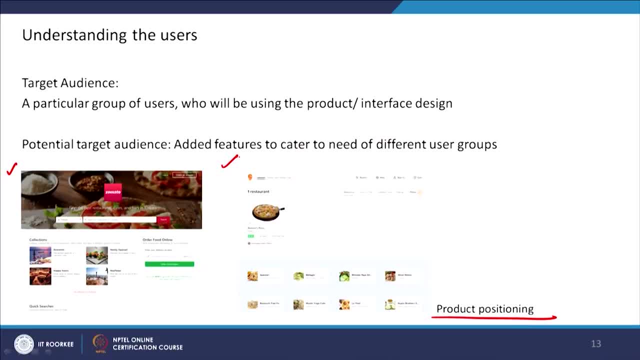 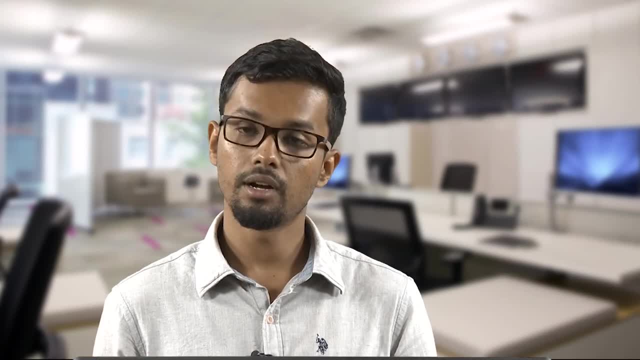 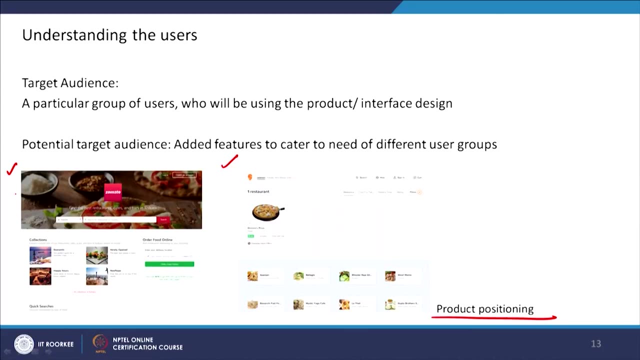 example, if we take Zomato and Swiggy, they perform right now they perform the similar task, But the way Zomato project the company and way Swiggy project the company, they are different Because Zomato, the first key features of Zomato is giving the review of the different restaurant and talking about the 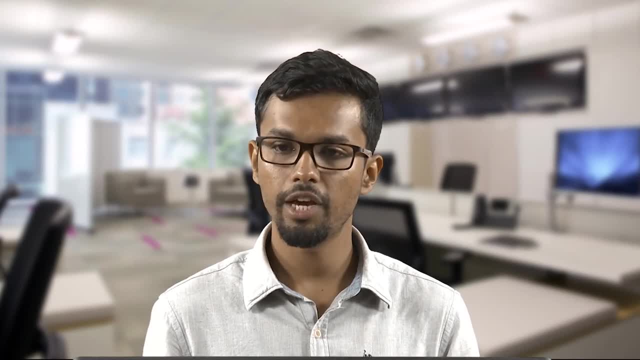 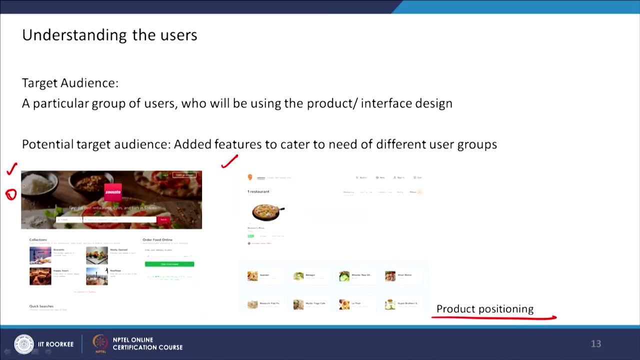 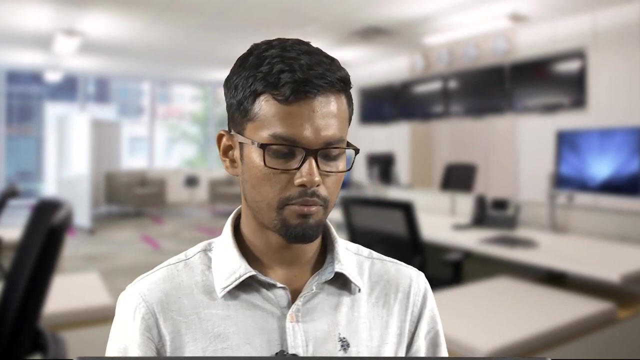 menu, what are the different chains and customer review. That is the first and foremost task of Zomato, and Zomato is designed like that. And then there is another part which is added, which is you can order food online if the possibility is there. But within Zomato, everybody knows that within that. 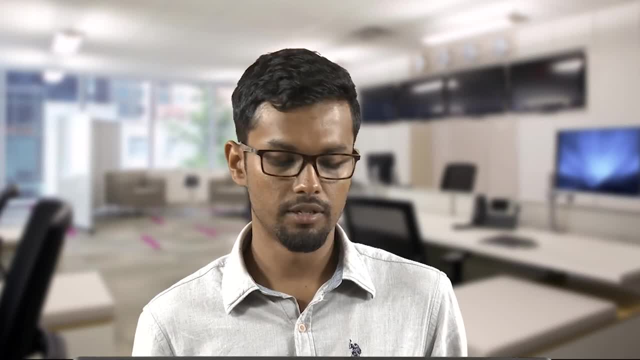 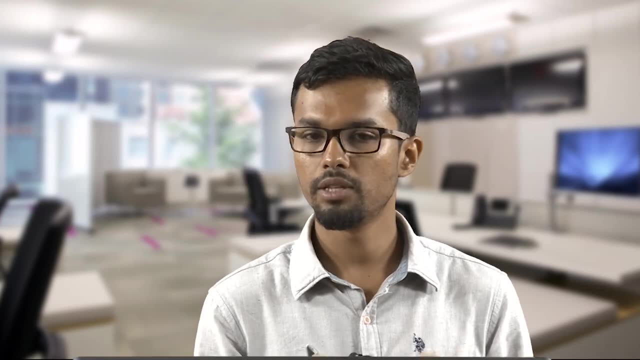 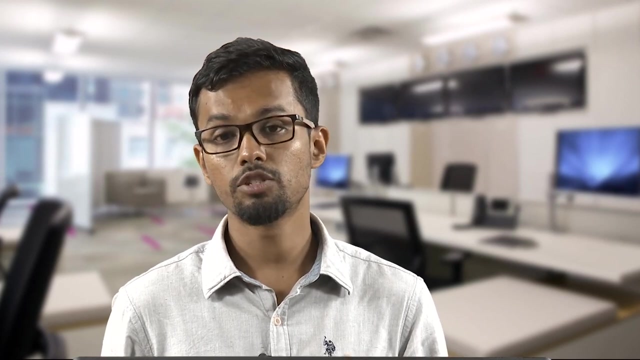 there will be lot of restaurant which will not give you the online order, So Zomato does not only cater to those who gives online order. So Zomato position themselves in a different way. So, based on that, the potential target audience will also change and the customers expectation from the 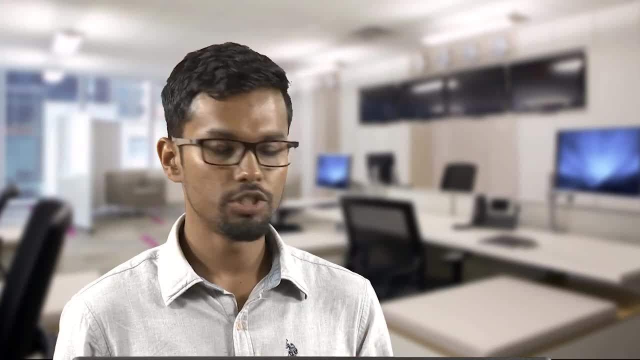 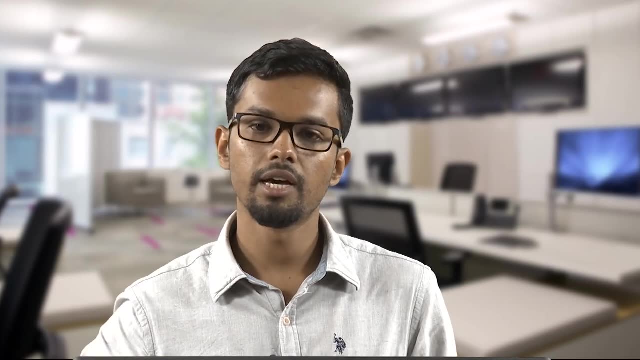 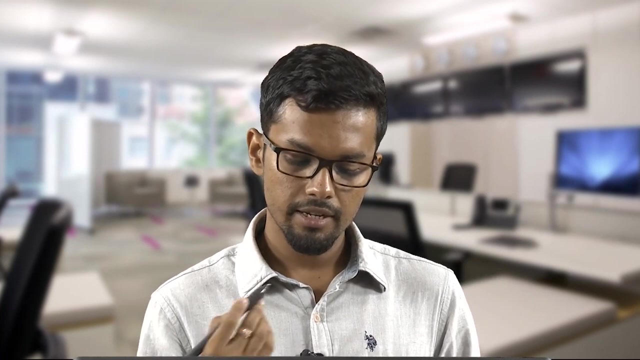 company will also differ, Because when they are launching in the Zomato website, if they are already acquainted about the Zomato company and their brand image, they will expect some different kind of task to be performed within this website. And then the Swiggy. on the other hand, their 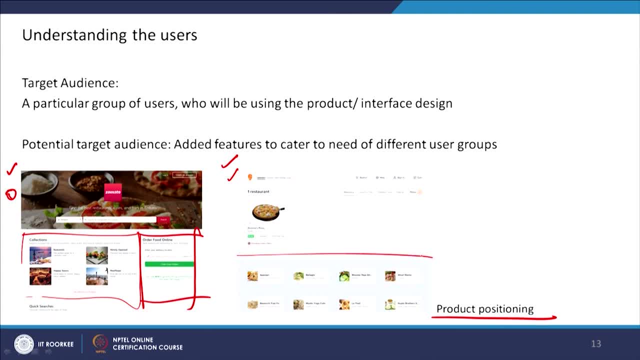 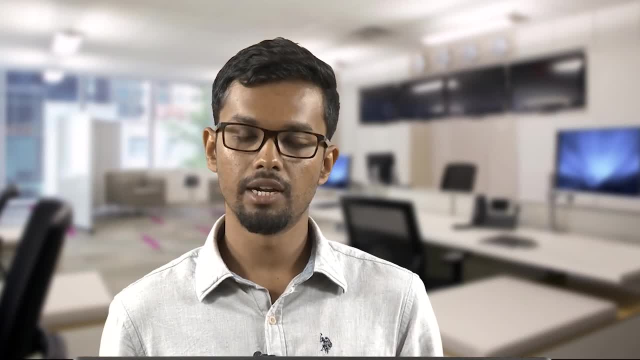 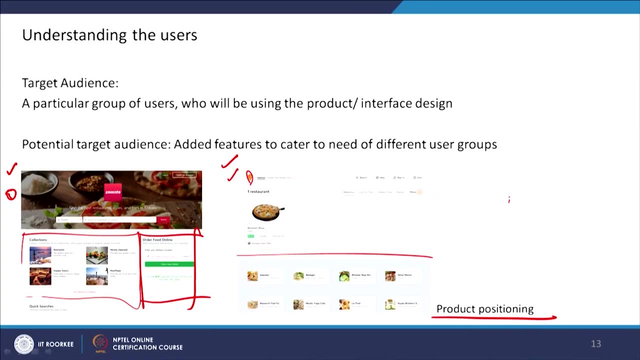 main thing is ordering food online and they will deliver it. So Swiggy also. that is their strong point: to deliver faster delivery, and that is how the company evolved to locate the so it is. their logo is also like this and which gives kind of an identity of location. 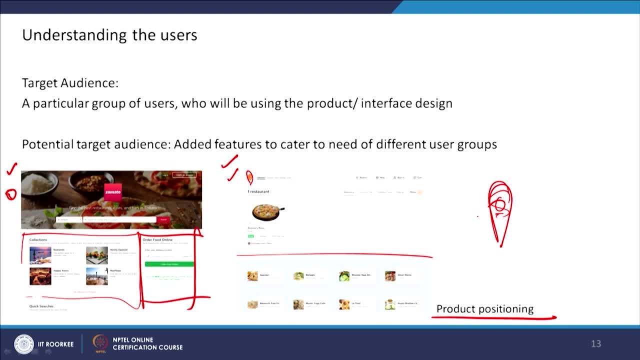 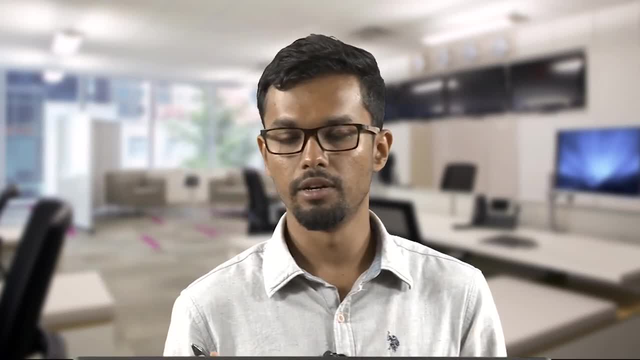 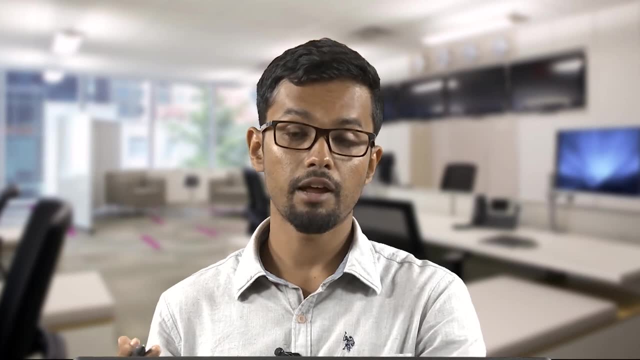 And wherever you are, so they will deliver the food. But now Zomato also performs the same task. Swiggy also performs, But Swiggy is more defined into only this kind of task, which they will just deliver. So that is how the expectation: they can be similar people when they 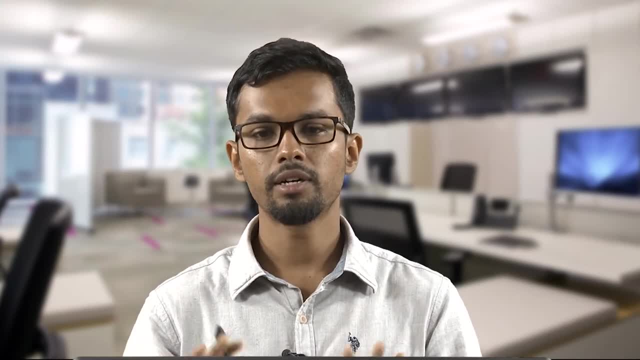 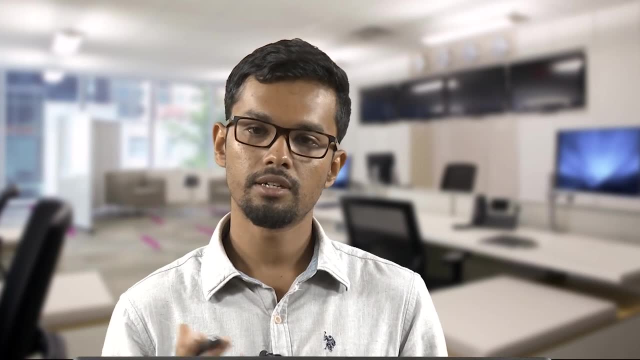 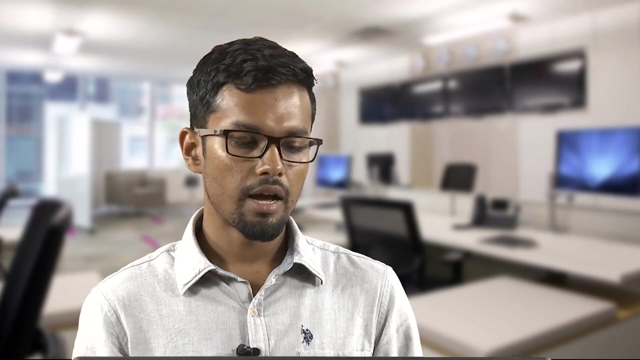 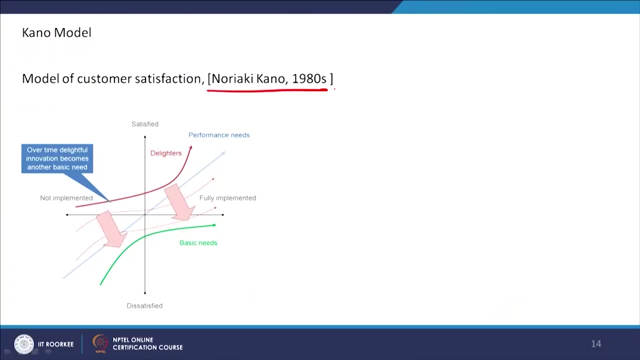 interact with the two different product. their performance, their expectation and their behavior will differ. So that is how the positioning also changes the target audience behavior and how this product has an image on the paper. And now let us discuss another model which is given by Noriaki Kano in 1980s, which is called Kano model and which is the 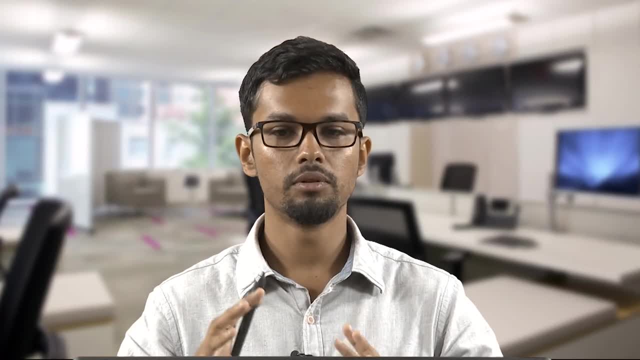 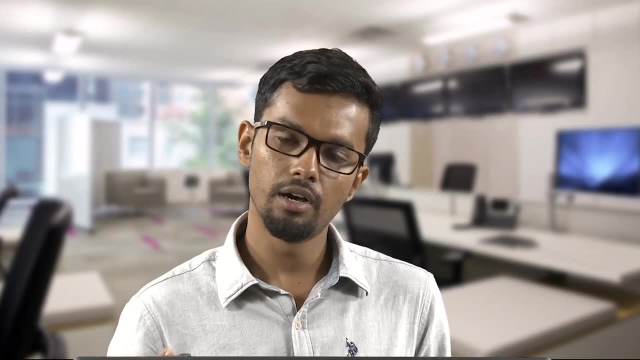 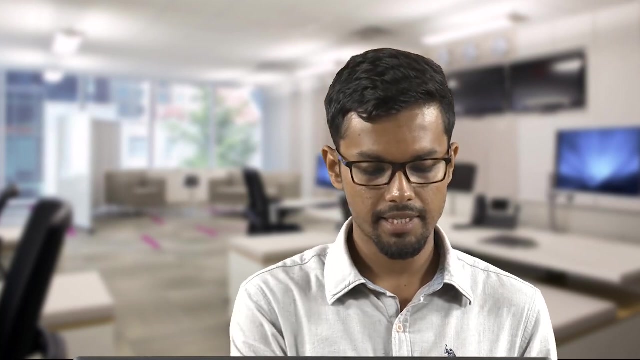 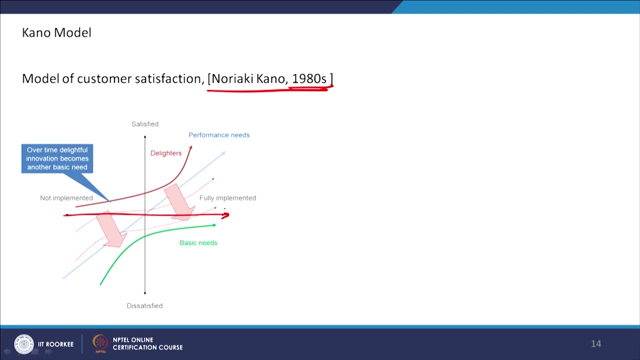 interface between the product and the customer and how their satisfaction level and the performance of the product and the satisfaction level of the customer varies. Now this model is there is x and y axis, So in this y axis this is portrayed that implemented features, not implemented features, to fully implemented features. So more and more features. 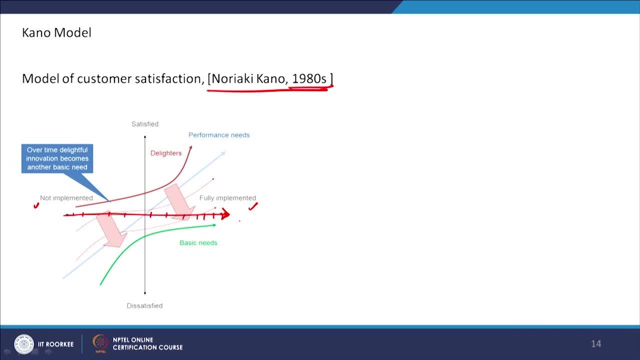 towards product is in this side, So more and more products are having the same features are on this side, So it can be the early mobile phones, It can be the new mobile phones. There are lot of features implemented within that. So this comes in this axis Now: satisfaction and customer. 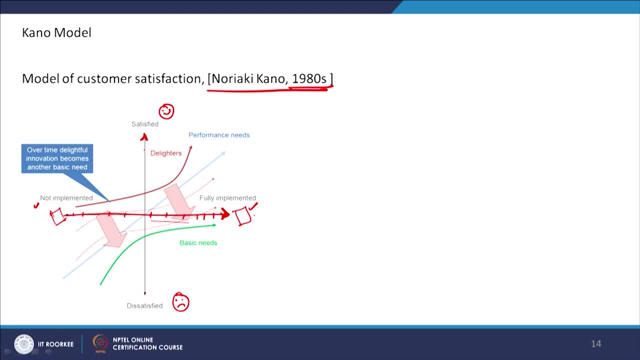 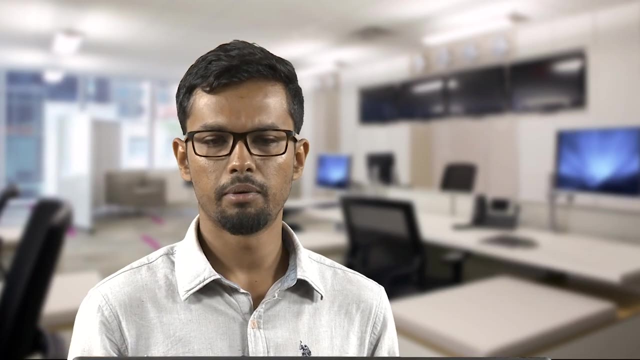 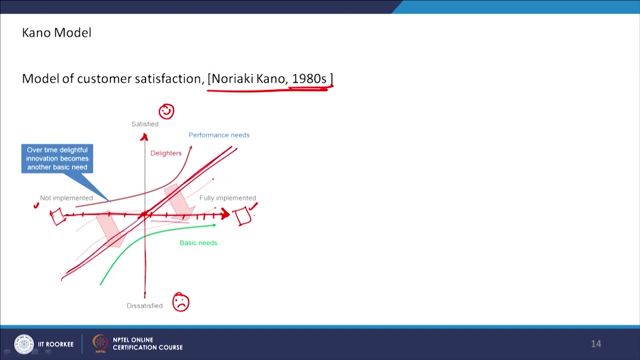 satisfaction and dissatisfaction is plotted in this direction. So it is 0.. So customer has a neutral opinion and then dissatisfied and satisfied. So this is the performance, for a bare minimum performance, if the product performs okay and neutral. So this will go through this line which is at few of the features. 50% features are implemented. 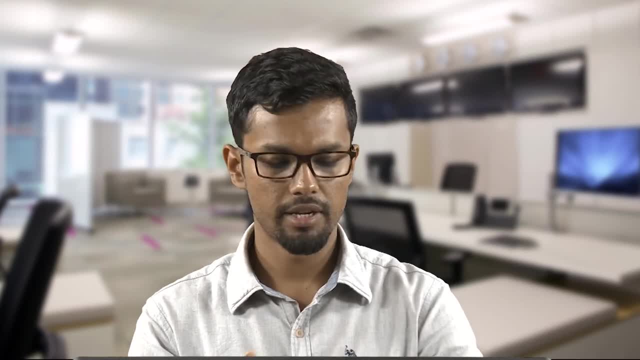 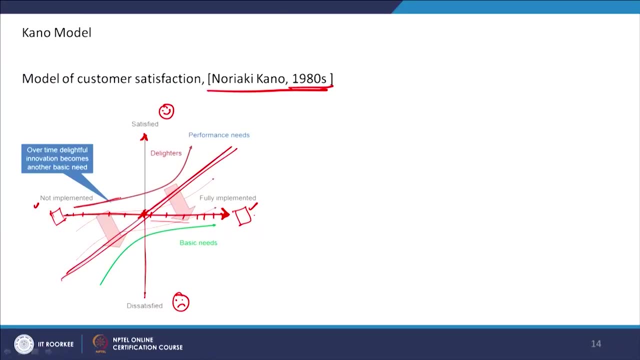 and customers are more or less satisfied And this is the performance of the product. So customer, it is not satisfied or not unsatisfied. Now this is if the product has more features. the features over here and this has the satisfaction rate is over there. So this 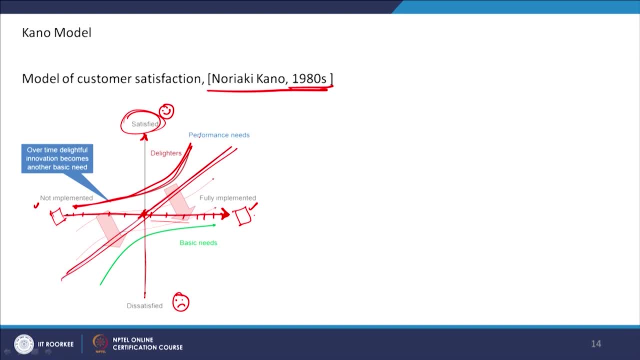 is called delighters, which will be above this line and where there are less process, less numbers of features implemented and less numbers also is performing well, So customers are satisfied. So this line is a delighters line when customers are delighted. Similarly, this line is a basic need or when the customers will not be delighted at all. 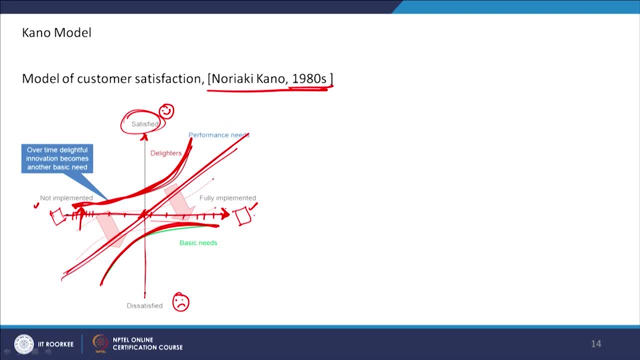 So this line is the bare minimal performance. otherwise the product will not even be sold. So features are less and then gradually, when this is going for the more and more features are implemented. still, customers are not so satisfied. So more features will definitely lead towards more satisfaction. 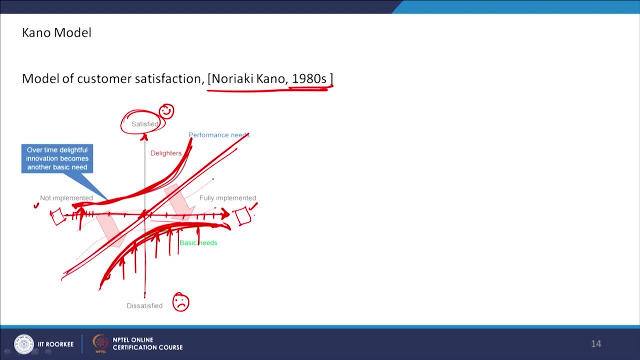 But still it will be on the same level, because features are not performing better, So performance is not pushing towards the satisfaction. So features are there, but it is leading, pushing towards the satisfaction level, but still this is not crossing to the basic need And over the period of time these delighters fall back and then they becomes the basic need. 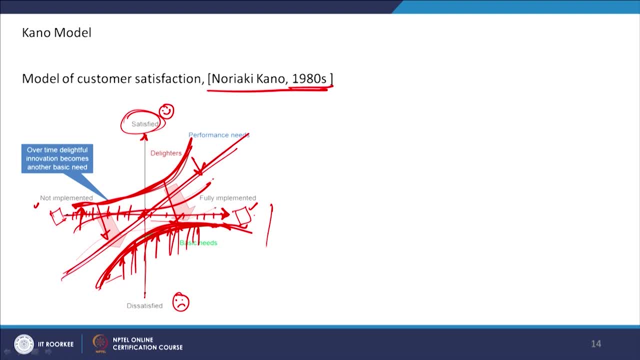 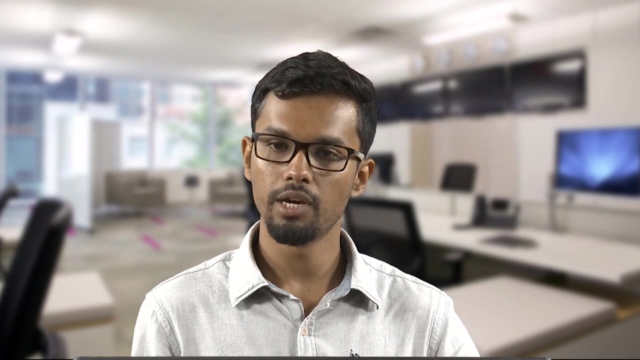 So more and more typology of more and more features are getting. if the features are getting implemented more, then these curves comes down and delighters becomes basic need. So over the period of time, if we see the, take the example of a mobile, So if right now we give the earlier versions of Nokia, 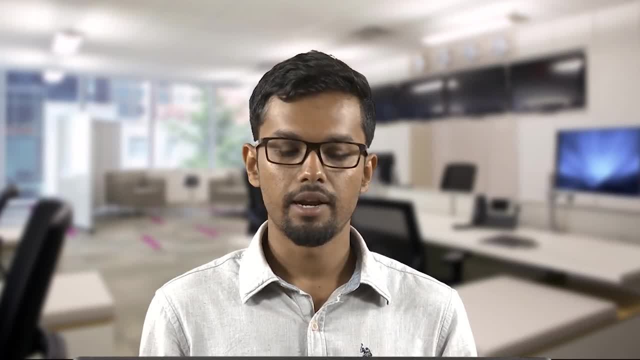 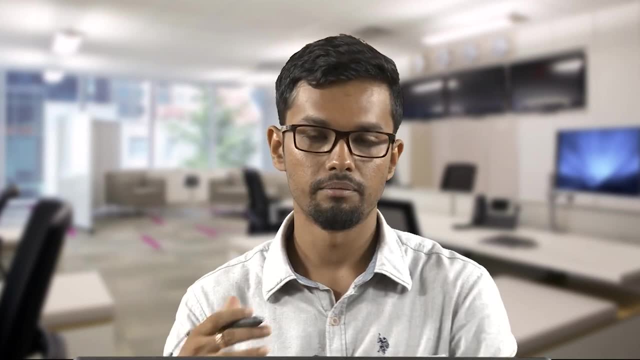 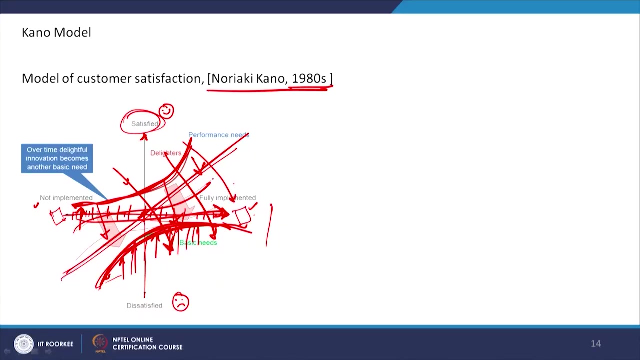 mobiles. So people will not be satisfied at all. And now we need more options, but in each and every options has to perform properly and then will be satisfied. So that is why the delighters are falling back within the need. So the basic needs what that time was, and so there. 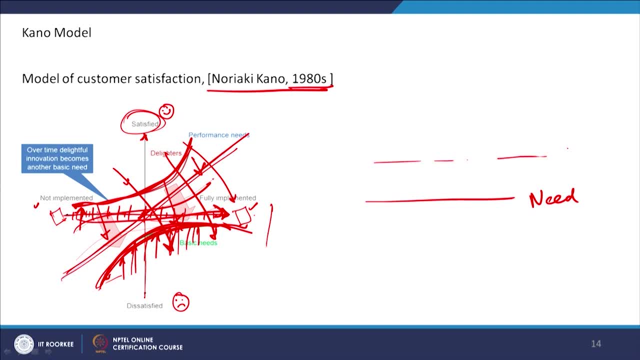 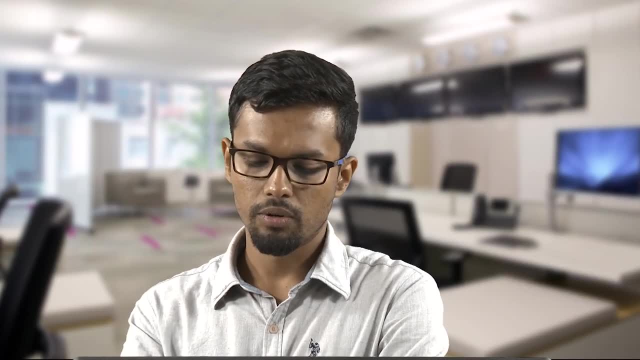 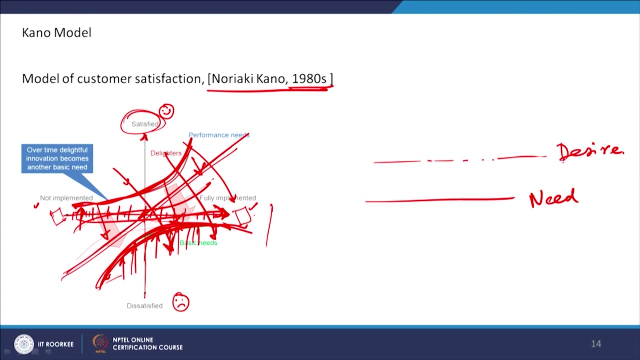 is a need, Okay, Of customer and this is a desire which customers wants but which is not the basic need. So over the time, this, when the desires are added in, the most of the competitive product. So these desires again comes as the need. So right now, the need of a mobile phone, which is the basic need of mobile. 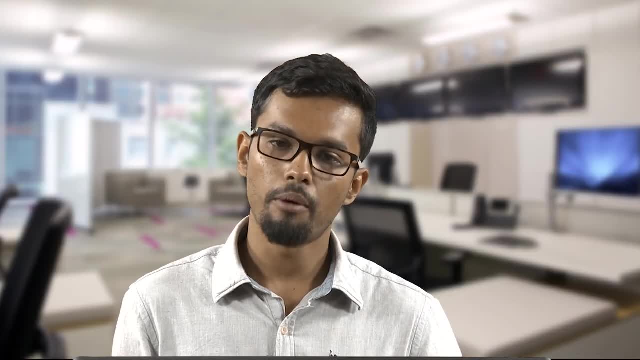 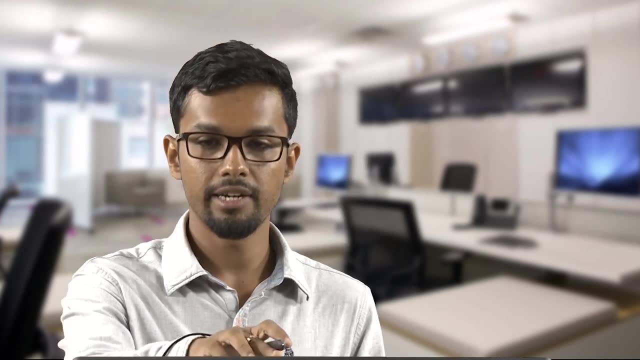 phone will. it will have whatsapp and facebook and other options, which becomes a basic need. and the camera is a basic need, right, And this is valued, to show that the desire is not coolized because of this car now, But earlier, in the earlier times it was not. It was added desire which customer wanted as a 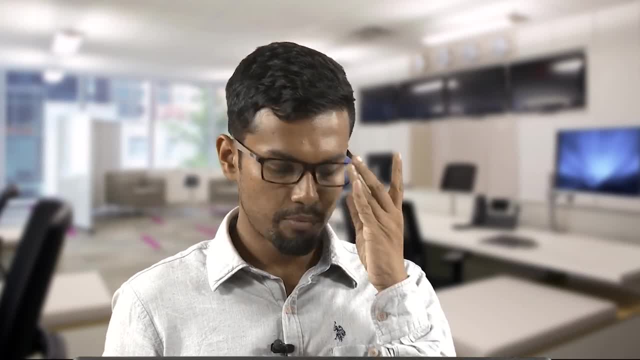 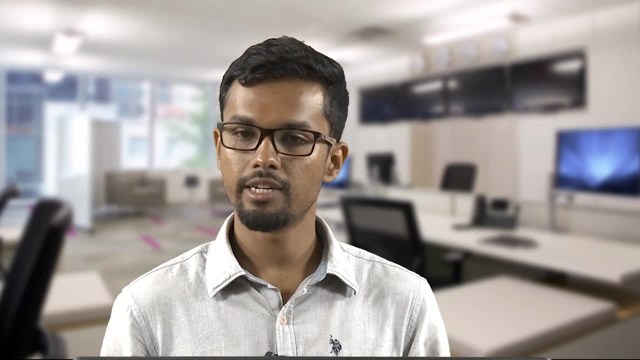 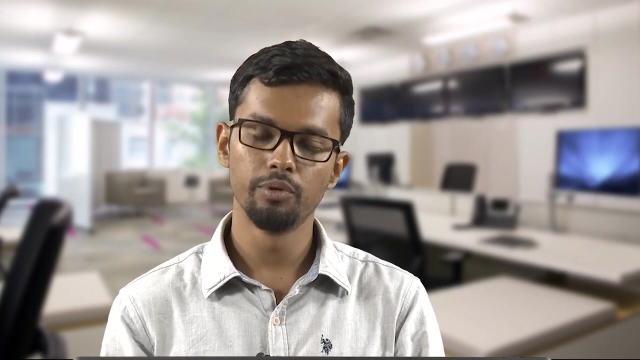 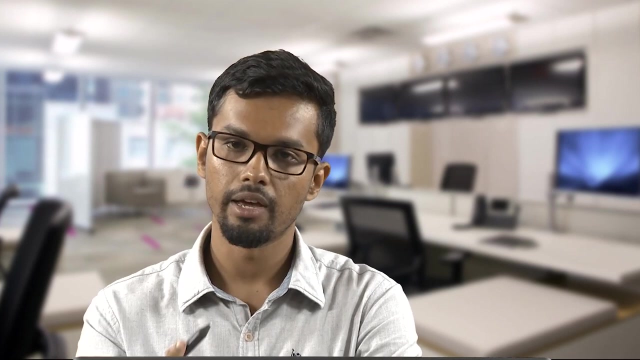 wish. Now that is how the product also has a particular life cycle. So if the product is not changing and the new features are not getting added and, based on the customer s users requirement, the product is not adapting itself with the users requirement, then the product will have a life cycle and it will end. So that is why regular testing and customer 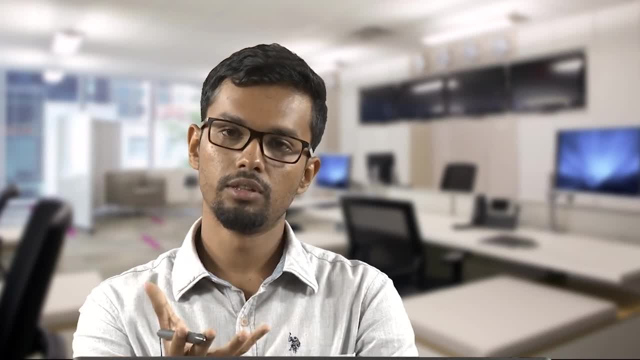 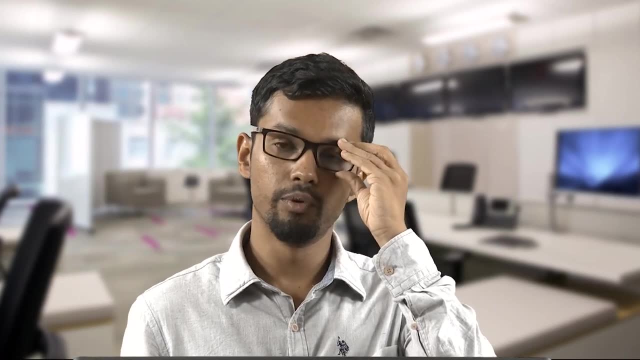 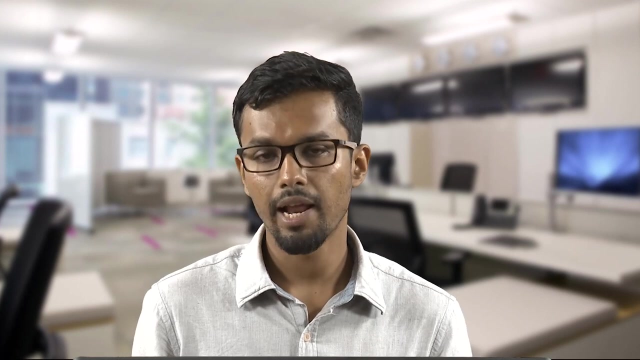 feedback, users, feedback opinion on the existing product and benchmarking with the other product. what other products are launching within the market? It can be product, can. I am using the term product, but this is in terms of this class. it is interface, So whatever. 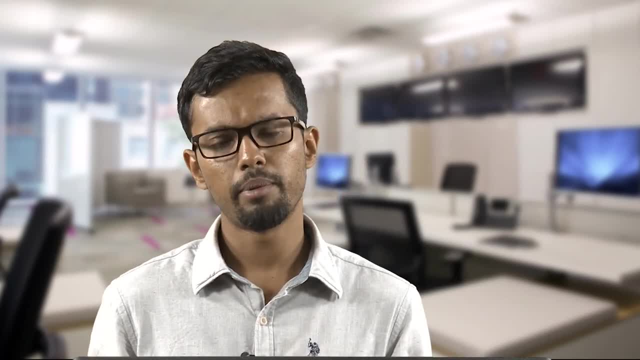 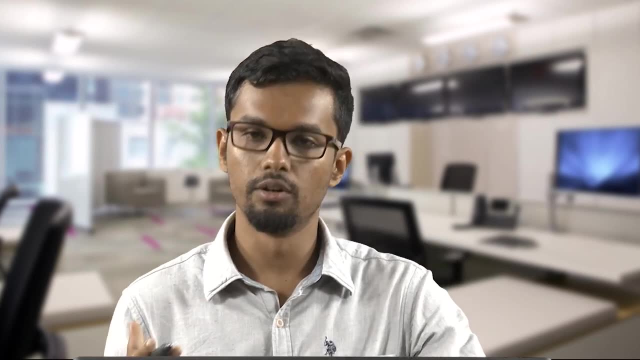 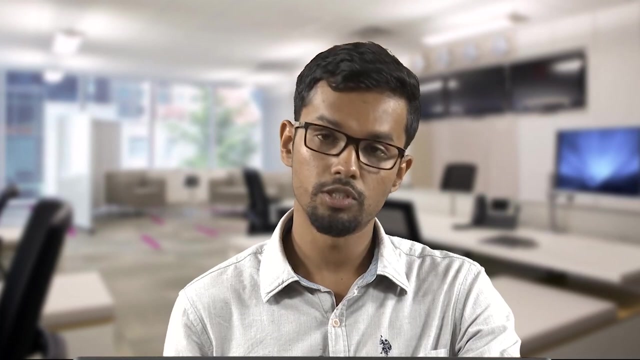 the interfaces web application we are launching. that web application has to have a benchmark with the other existing web application which are performing the same task and also it has to update based on the requirement of the customer. So customer requirement also changes over the time, So that has to be catered to. So 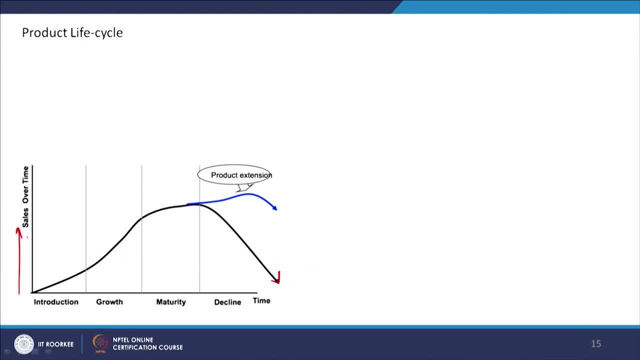 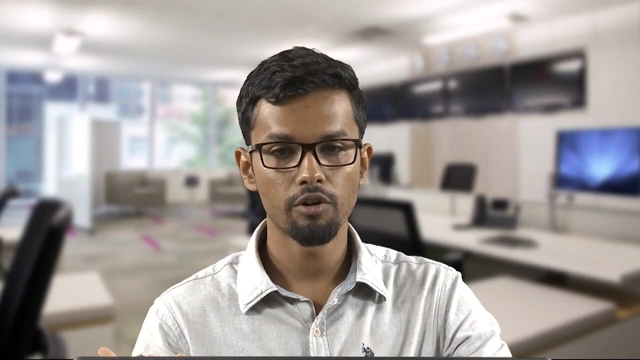 the sale overtime or the more the number of the people using the website. and this is the time, is the timeline. So first it is introduced, few of the people will be used, and then there is a growth rate when there is a marketing started and they will be more through word of mouth. or the few. 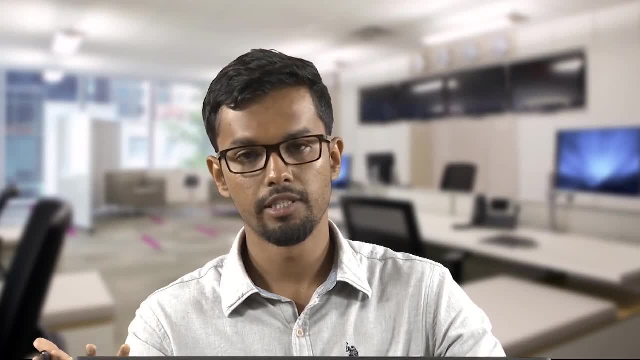 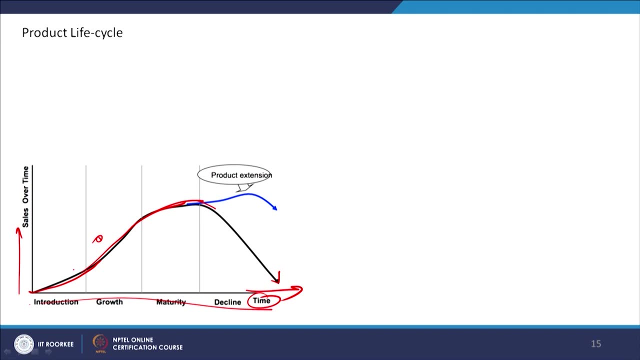 people who will be using. they might tell the next set of people. So there is a growth phase and after that, when there is a no change of the product- we are talking about one single product, when there is no change, So it will fall down. So that is why the new generations of mobile phone 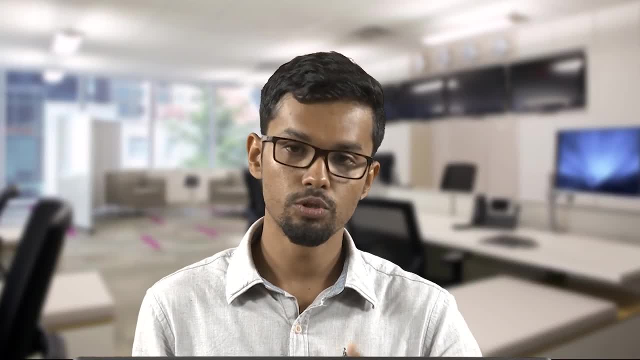 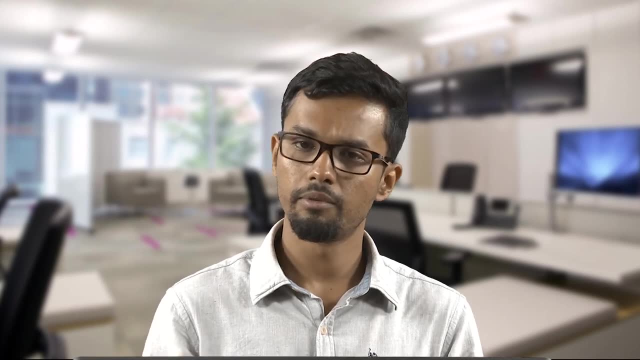 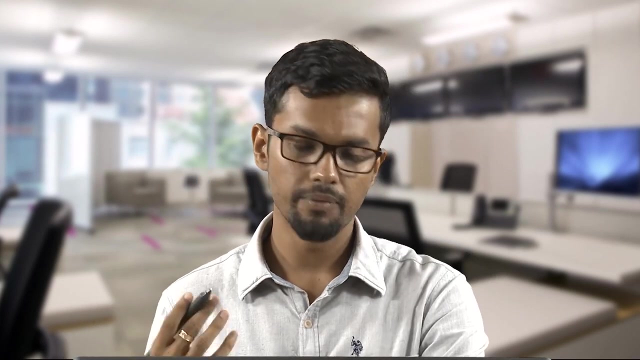 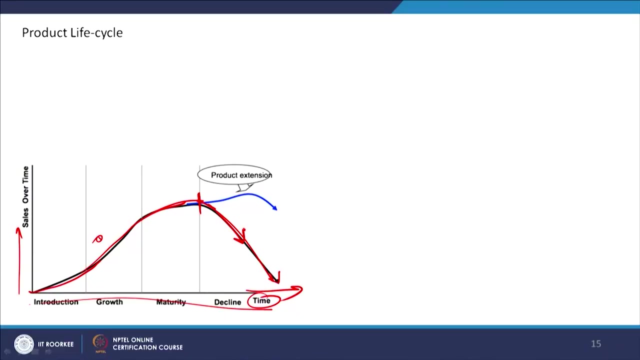 other products and website also changes its look and different features get introduced within the website. For example, Facebook introduced their timeline and it always they try adding new features within different websites. So here when it starts to fall down. so designers and management, people should envision that, should be aware about that when there is 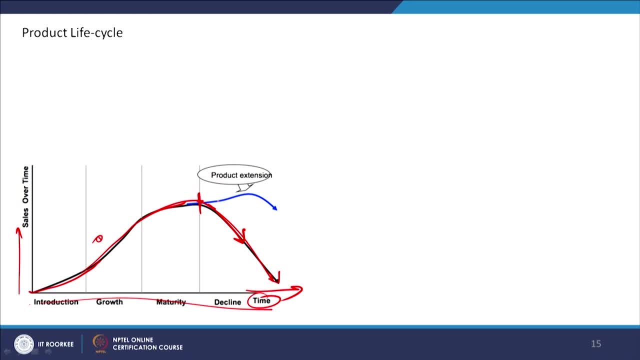 a growth rate that is there. So that is why we are talking about the growth phase. So that is why customer s expectation and the product s performance is not matching. So the product has to be extended, or product should change their features and then another curve will start. 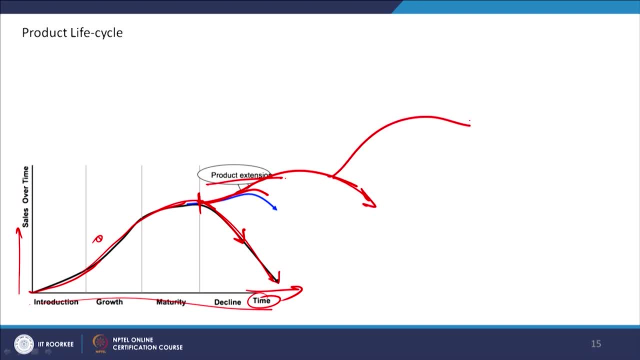 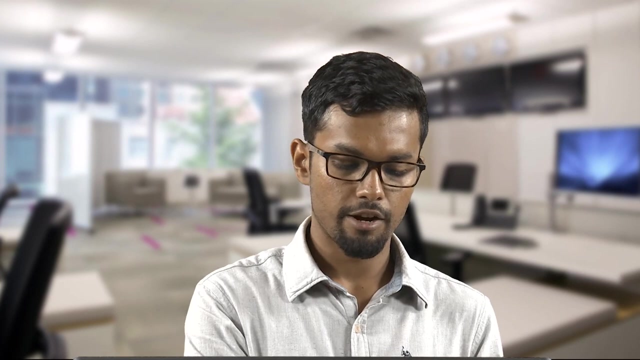 And then when again it is falling back, then it should again shift, add some features or change, iterate or modify the features for a steady growth. So based on product life cycle. because of this kind of users, acceptance of the technology or the new product or new website, this kind of 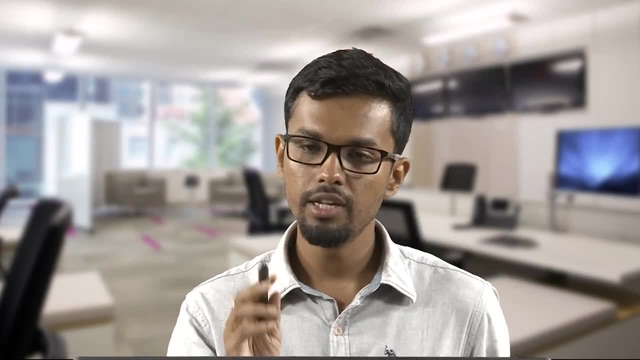 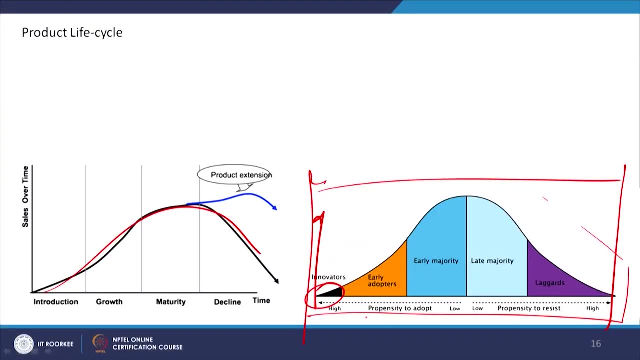 fallback also happens. So, first the innovator only. it is confined within the innovators or the designers. They only use that And, based on the propensity of the adoption, the early adopter uses the new features of new websites, new web applications. 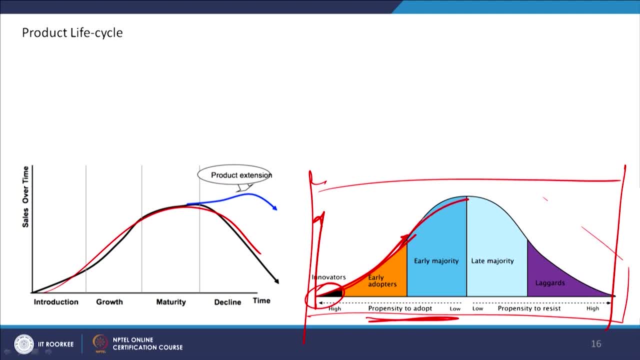